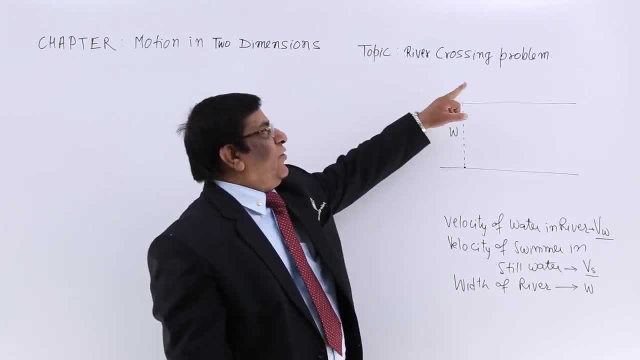 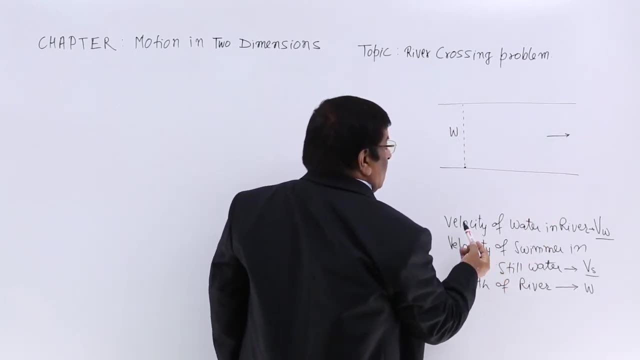 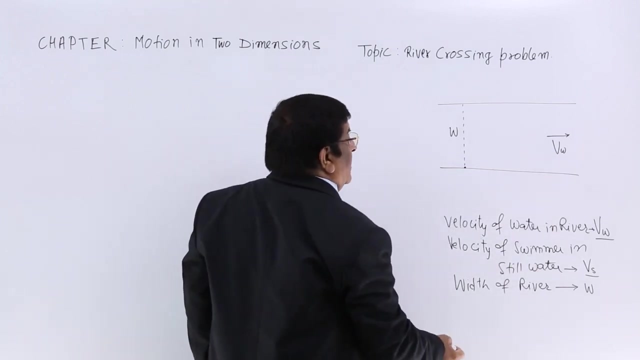 There is a problem, a very famous problem: river crossing problem. This is a river. Water in this river is flowing in this direction. The velocity of water in the river we will take as Vw. There is a swimmer on this side. When he is in the still water he can swim. 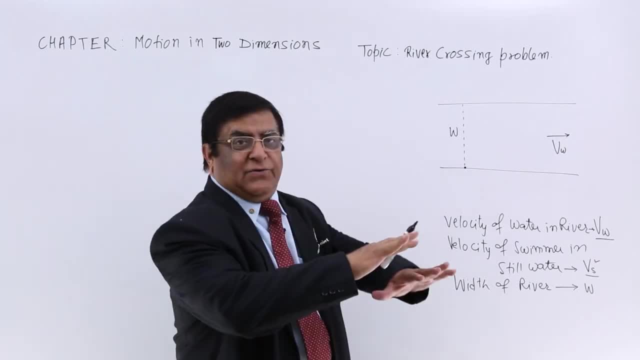 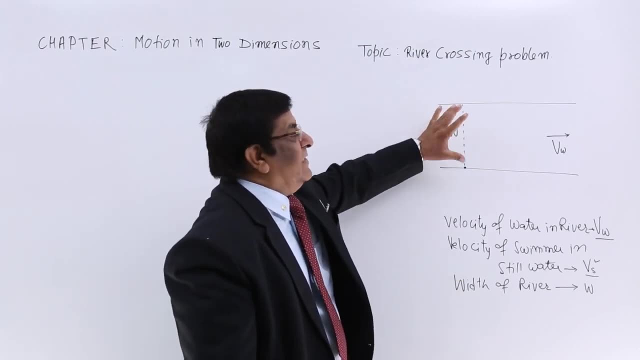 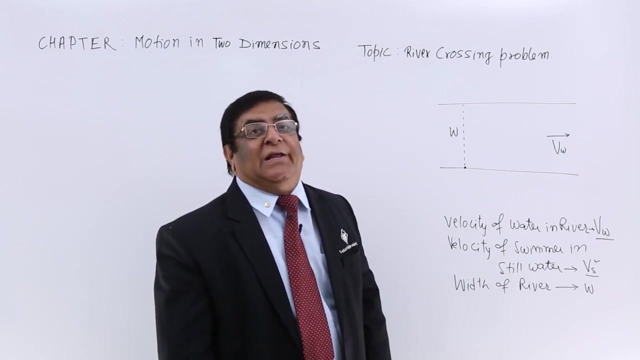 with a velocity Vs In a swim water. in a pond he can swim with a velocity Vs. ok. Width of the river is w. Now he has to cross the river And we have to find out how much time will take And where will he land up. There are two type of crossing the river-. 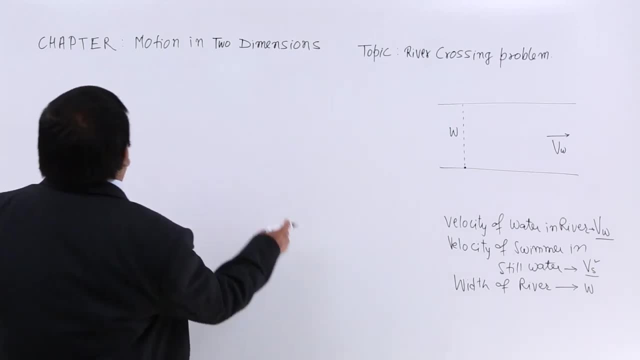 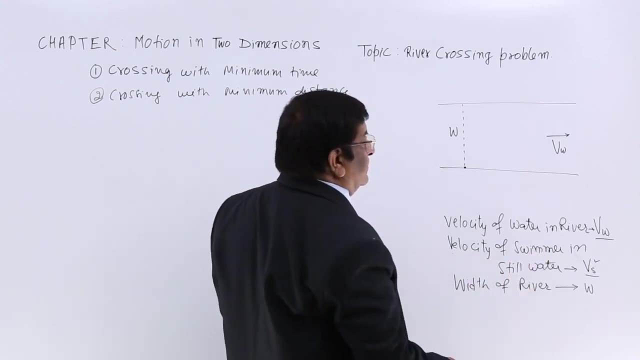 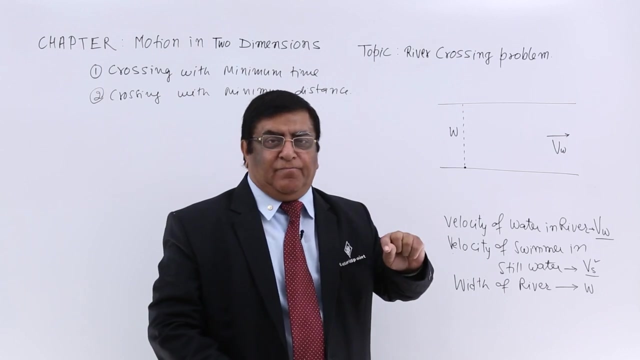 one with the minimum time and one with a minimum distance. Now he is is making efforts to swim. the velocity of the swimmer in still water that means he is making efforts to swim and while swimming he has a certain velocity. that velocity is 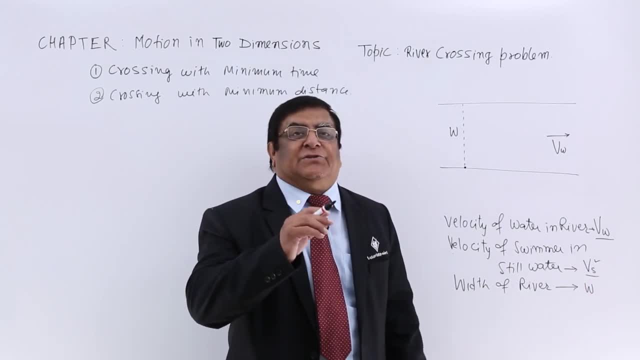 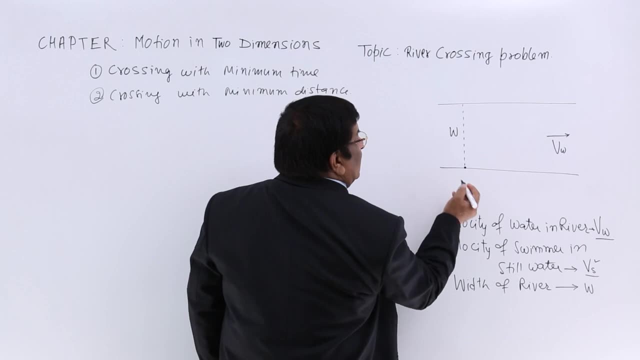 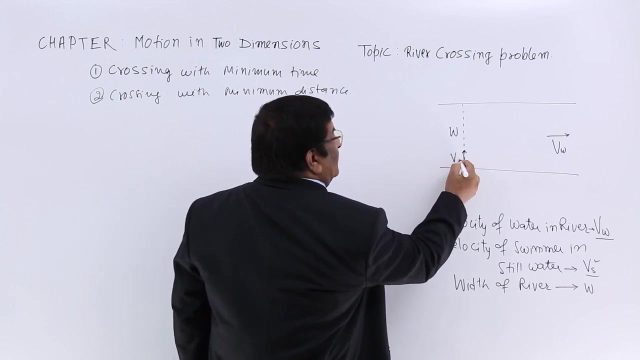 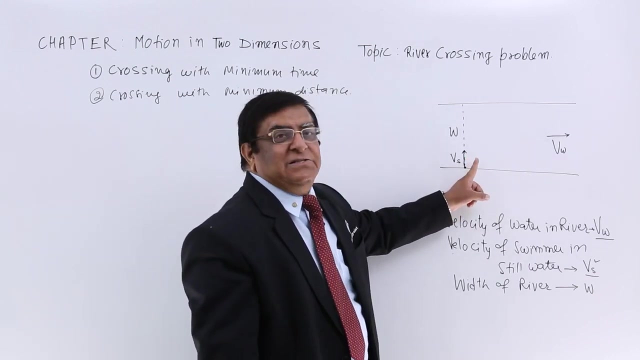 Vs, and this velocity has a particular direction in which he is putting his effort to swim. Now, if he is putting his efforts to swim in this direction, then his velocity can be referred by a represented by a vector, and this vector is Vs The river. the moment he is in the river, the water of the river is trying to take him. 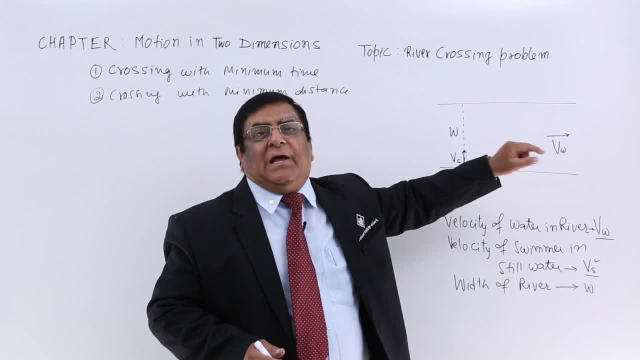 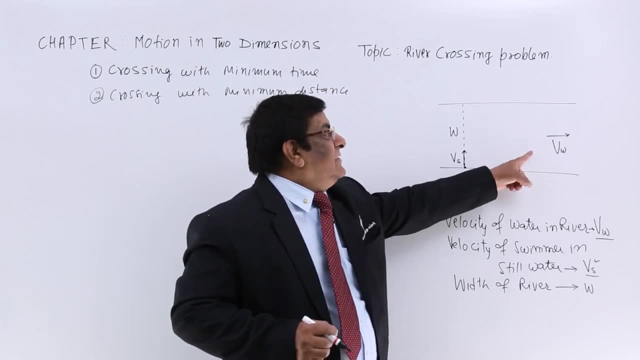 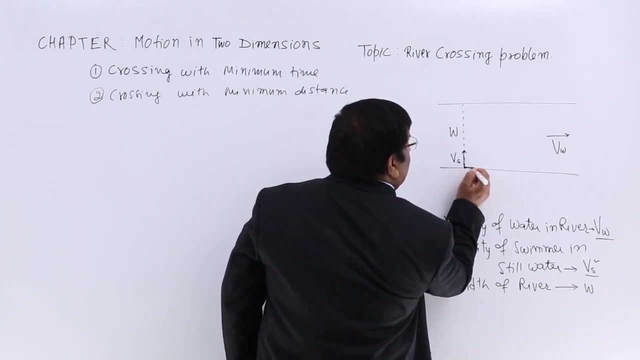 along the river, along the water, and that gives velocity to the body of the swimmer, whether he wants it or he does not want it. this velocity has to be there because he is on the water. So this velocity, Vw acts on it. 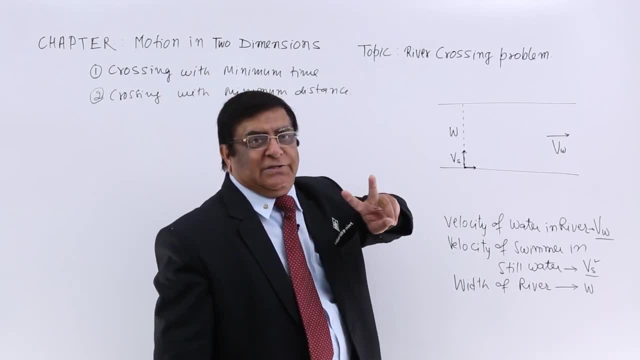 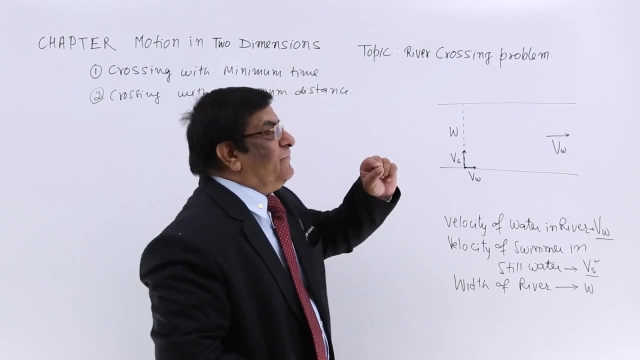 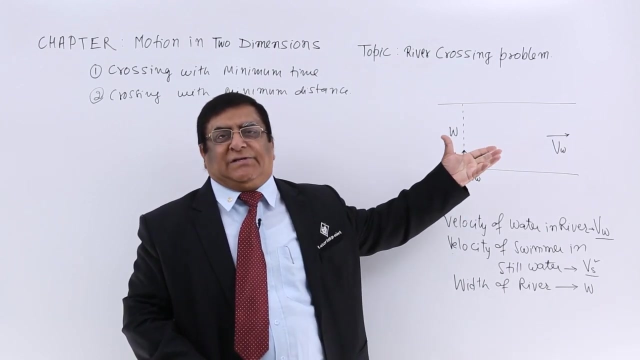 Now this person in the water has got two velocities: one because of his swimming and one because of the water. So if there is one object under the effect of two vector quantities of the similar nature, then what will be his velocity? The answer: it will be addition of the two resultant of the two, and we want to, we know. 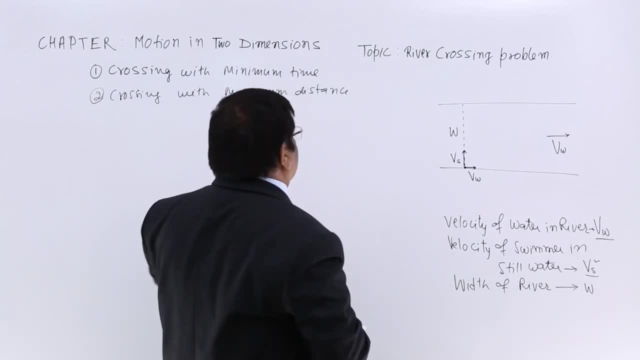 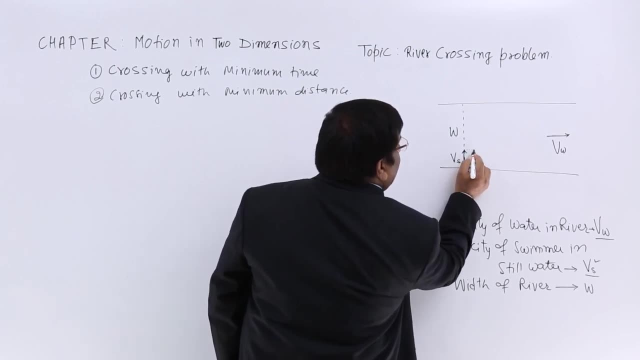 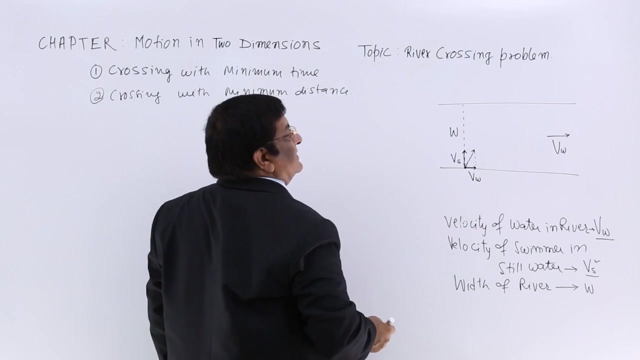 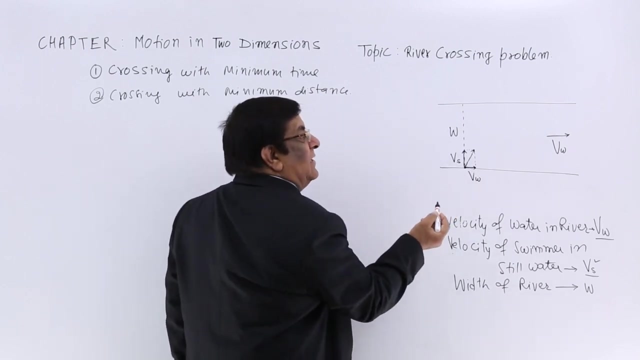 the method to find out resultant. So, to find out resultant, we complete a parallelogram, make a diagonal. this, this is diagonal, So he will be neither going in this direction nor in this direction, but he will be going in this direction. 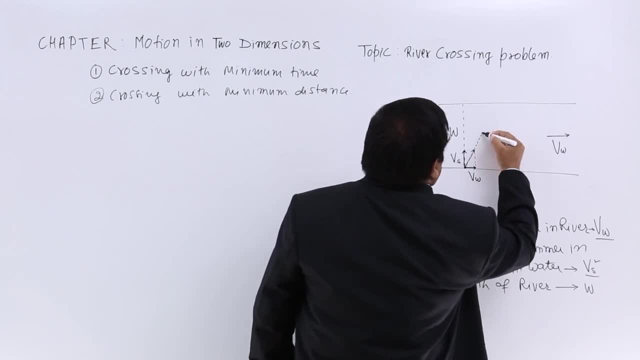 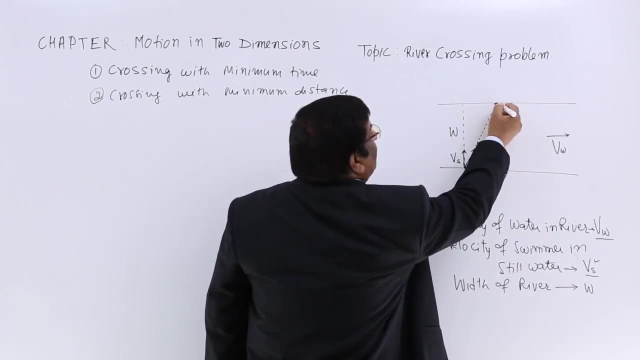 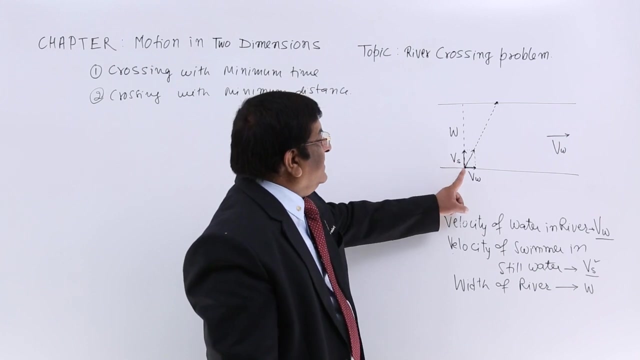 And he will keep on going like this, So he will keep on going like this, So he will keep on going like this And he will land up at this point. So he is trying, he is putting his effort to move in this direction, but he is finally. 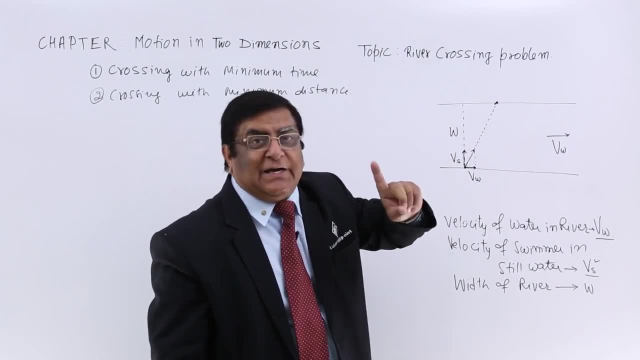 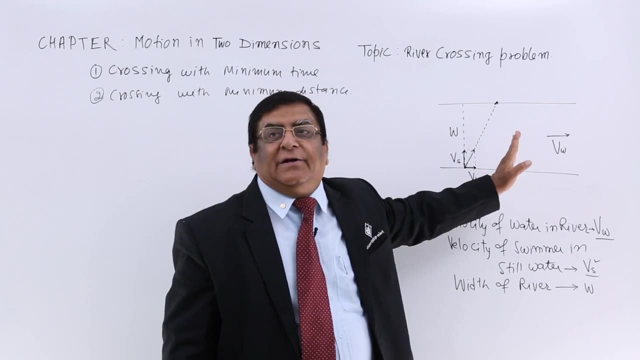 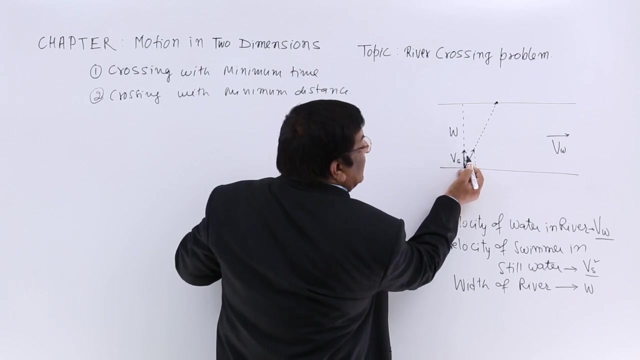 landing up in this direction. So for all the time he is swimming in this direction, the water is pushing him down the river. So he will constantly fall down the river. So when he travels up to this much, the water push him here. when he goes here, the water. 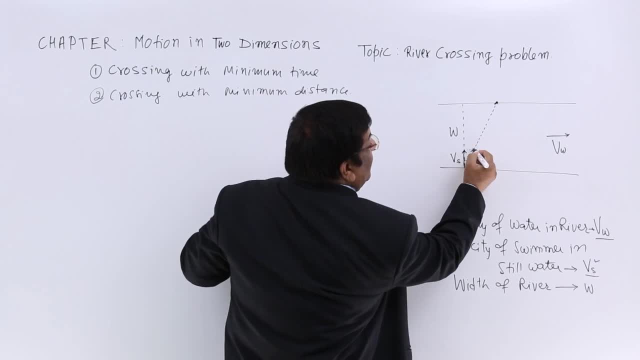 push him here. when he goes here, water push him here. when he goes here, water push him here. when he goes here, water push him here. So what happens? He is either here or here, or here or here, under the effect of both the velocity. 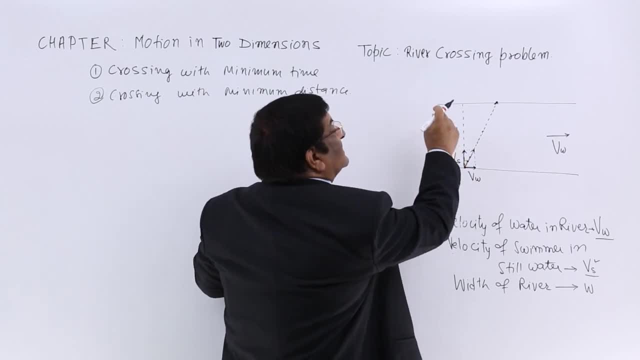 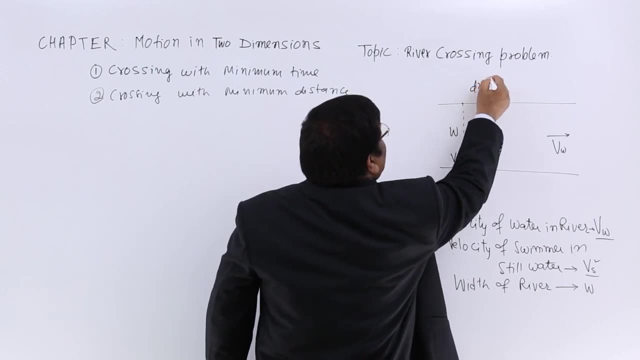 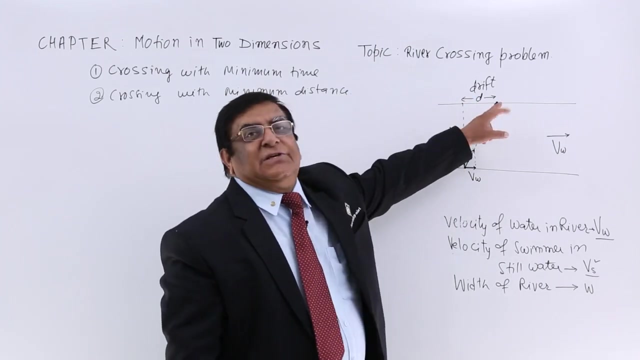 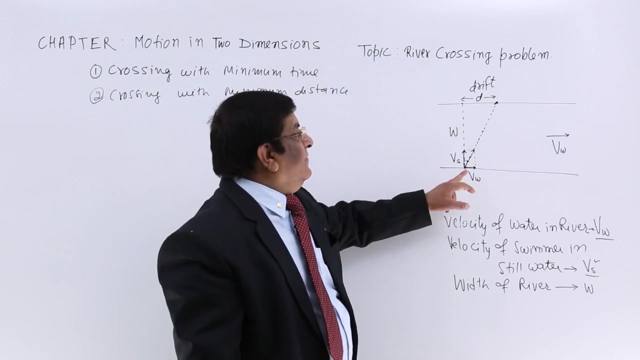 So this is what happens to him and that is why he has drifted, And this will happen. So he will be drifting and this distance is known as drift D. This is this will happen if he is putting his effort to this point, which is just opposite to this point. let us give them name. 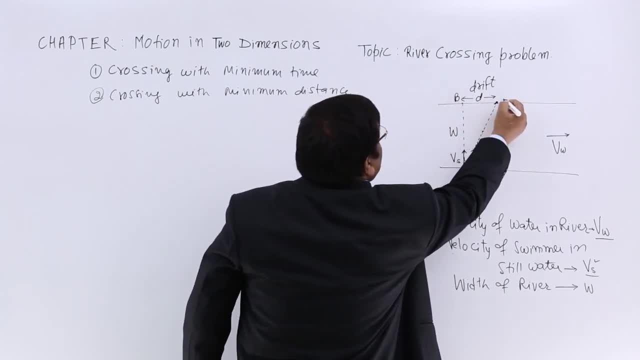 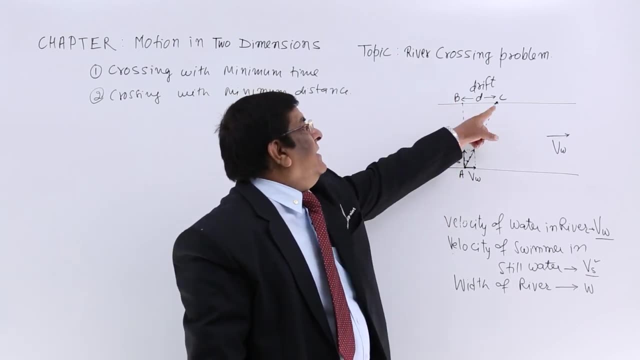 This point is A, this point is B, this point is C. So he is trying to swim in the direction AB, but he lands up at C. Why? there is a drift Because of the velocity of water. So this is the simple situation. 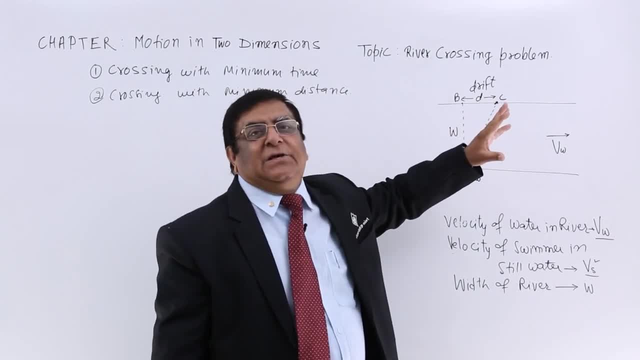 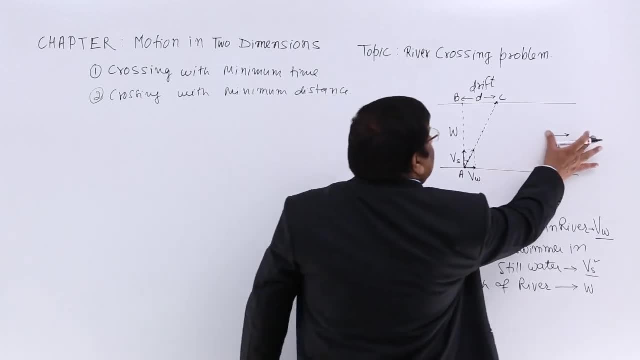 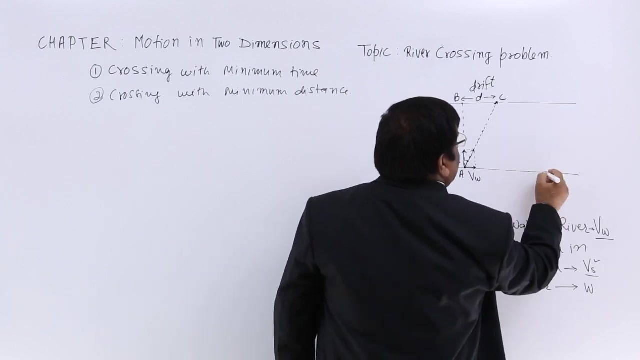 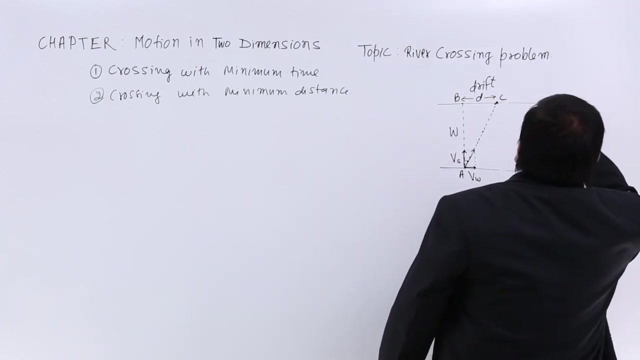 Now we have to find out which is the other way. if he wants to reach at this place, If he wants to reach at this place, I will create that situation here. Now he wants to. he is here and now he wants to reach. just opposite of it. 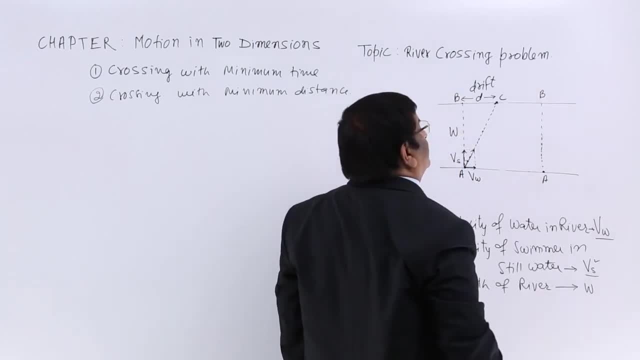 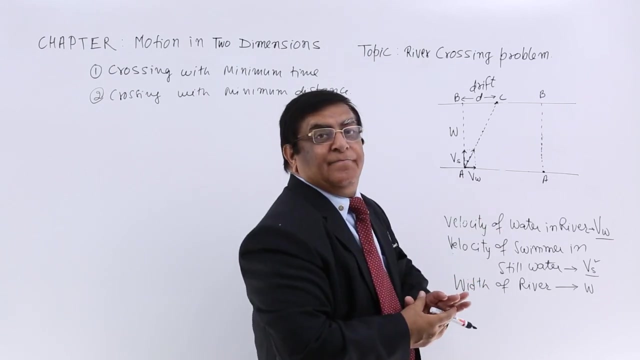 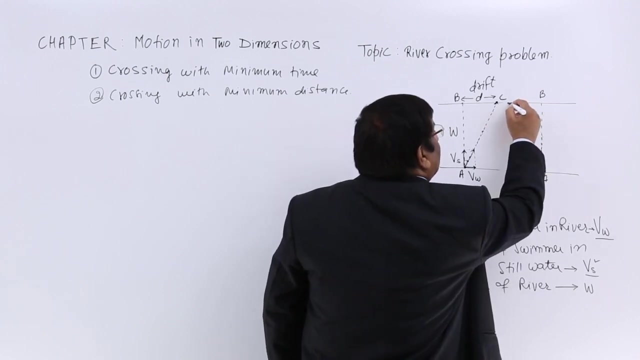 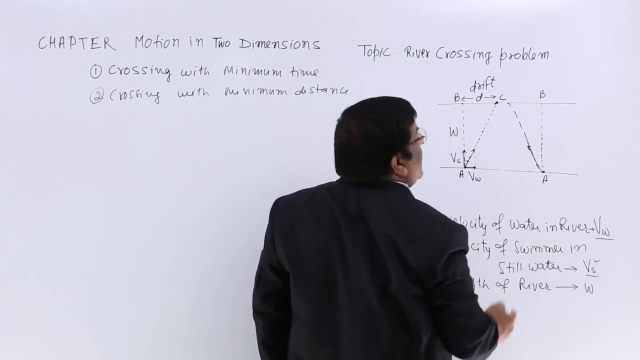 He wants to reach at point B. What he does? He try to swim in this particular direction. This is the D, This is the drift when he is in the water. So he try to swim in this particular direction. So he is swimming in this direction. 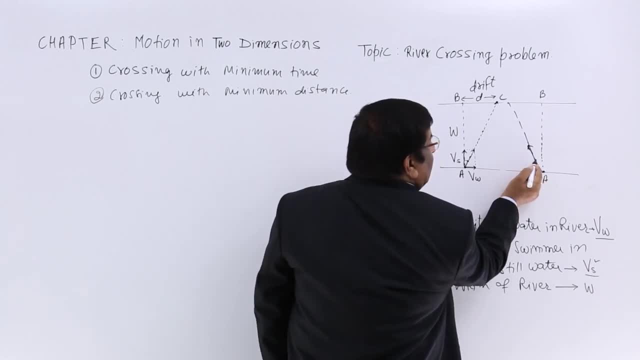 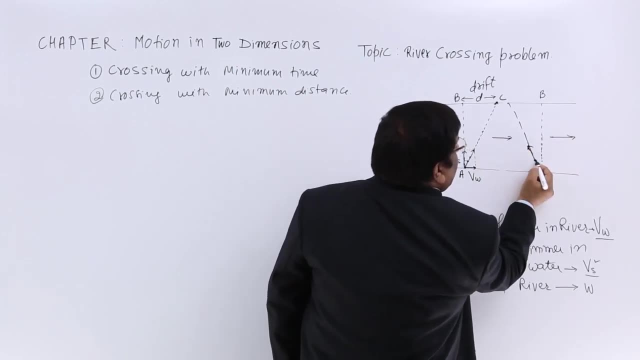 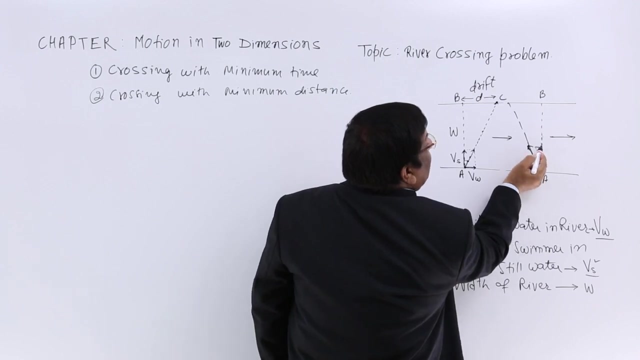 Now what happens to C? When he goes from here to here because of his swimming, the water is pushing him in this direction. Water will push him here Again. he travels in this direction. water push him here Again. he travel in this direction. water push him here. 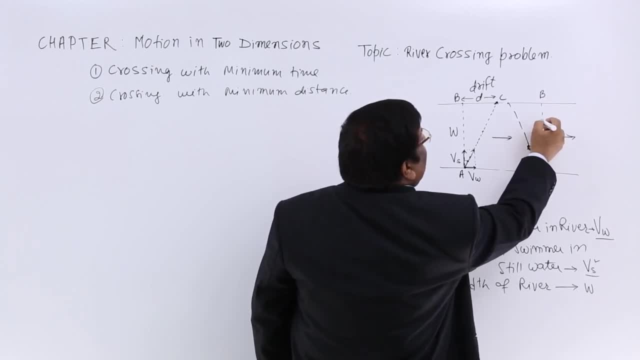 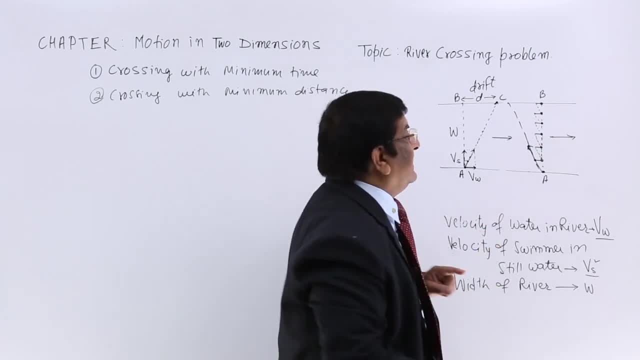 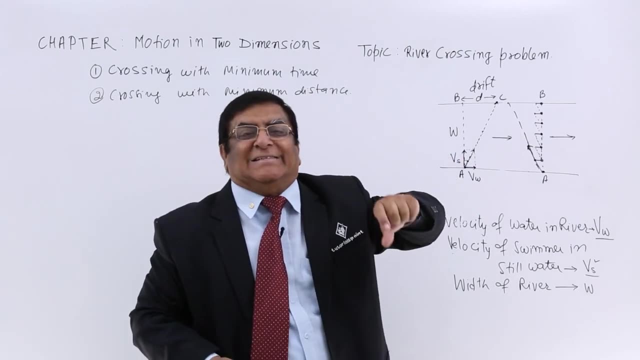 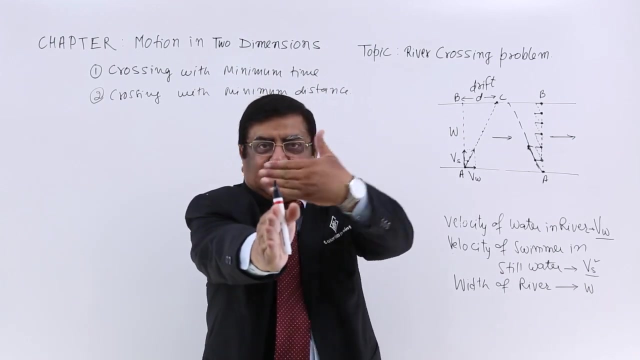 He is going straight, But all the time he is trying to swim in this direction. This is what happens when a boat man, a steamer man, tries to take us across the river. If he has to reach here- the water is flowing like this- then he will target this. 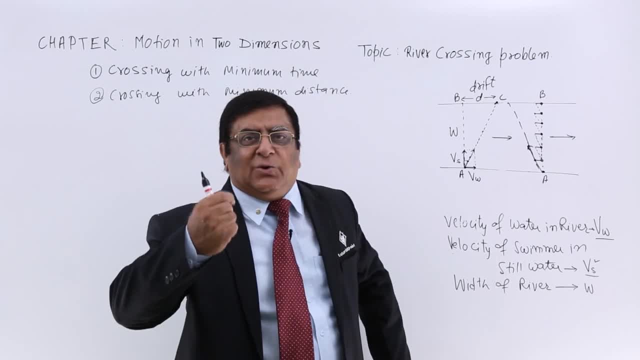 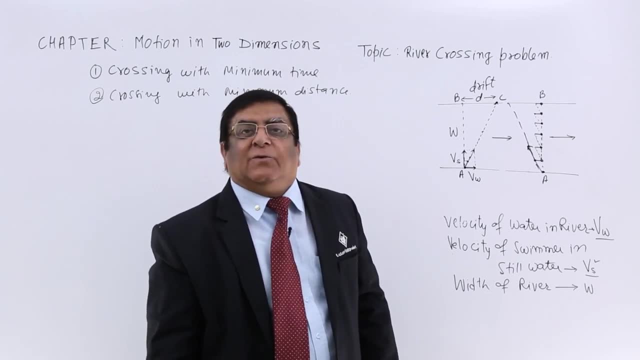 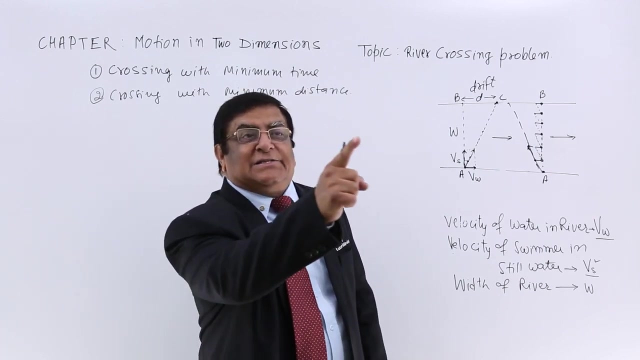 Why? Very simple: He knows that for travelling it will take 5 minutes. Why 5 minutes? In 5 minutes, water will drift him. Water will drift him 500 meter. So he targets a point which is 500 meter on this side. 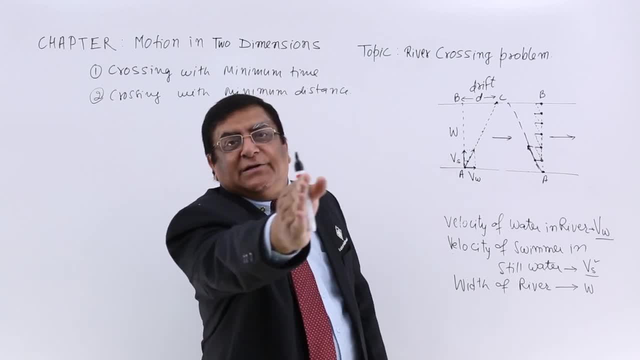 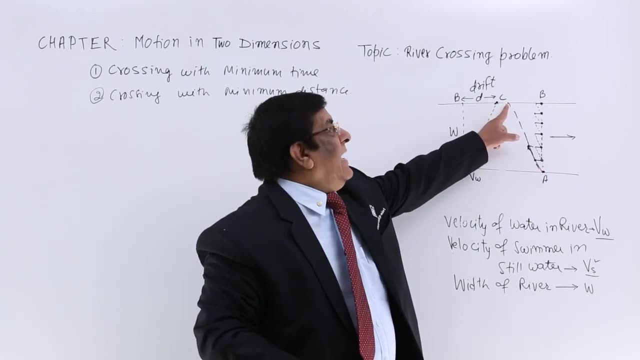 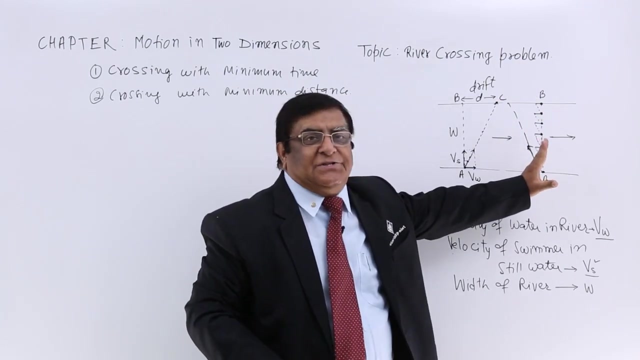 He targets and moves there, The water will drift him 500 meter and he will reach here. So he should target this point and he will reach this just across the river. Okay, Now, these are the two situations. We will analyze these two situations. 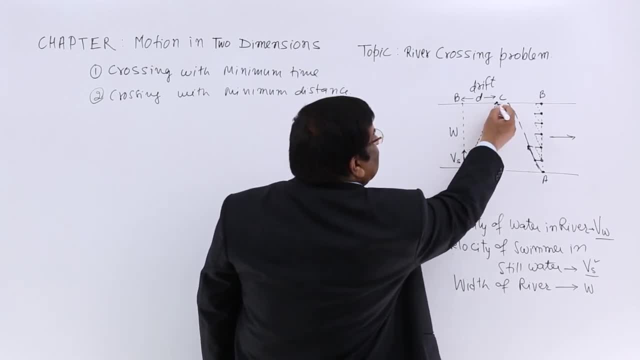 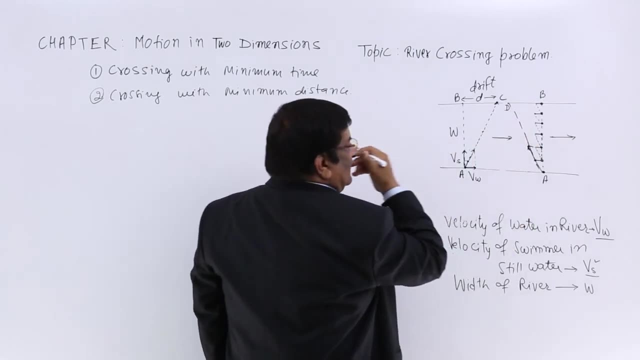 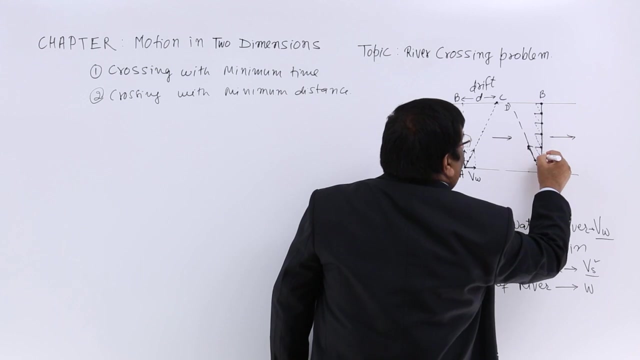 First, here, what is his path? His path is A to C. Here, what is his path? A to B, and he has targeted this point. Okay, This is his path, actual, and here, this is the actual path. Which of these two is his path? 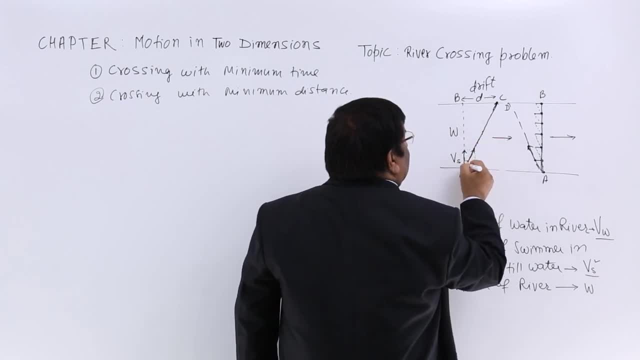 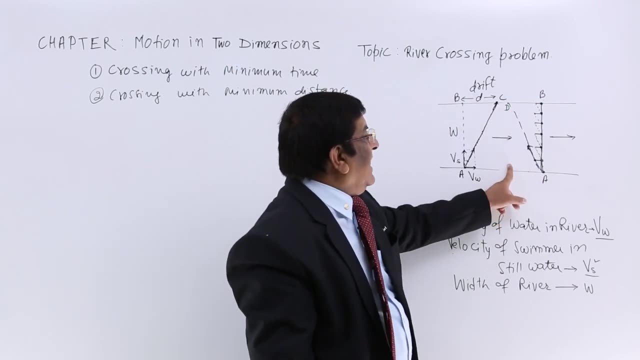 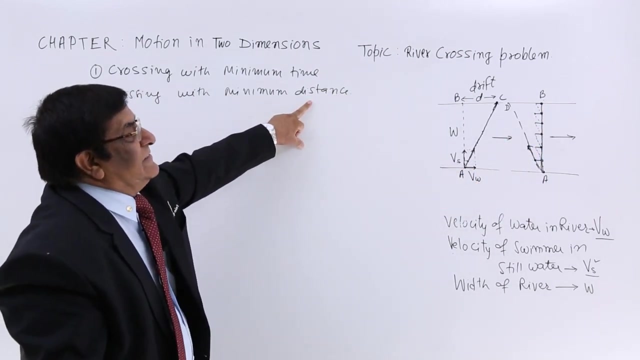 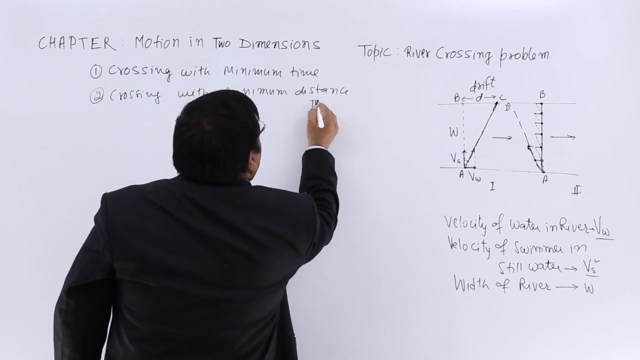 This is his path. Okay, which is the long, longer path and which is the shorter path? answer: this is the shortest path, so this is the style of swimming which will take him along the shortest path. minimum distance: this is situation number 2. this is situation number 1. so if a person is trying, 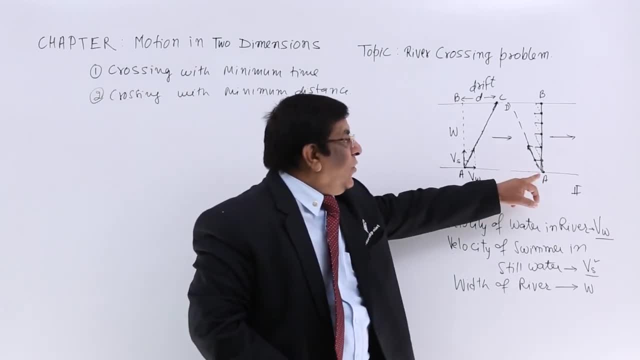 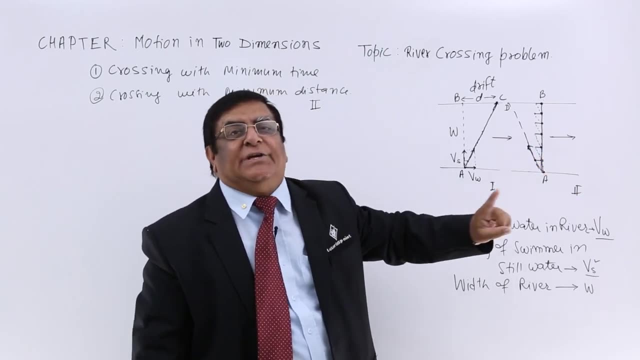 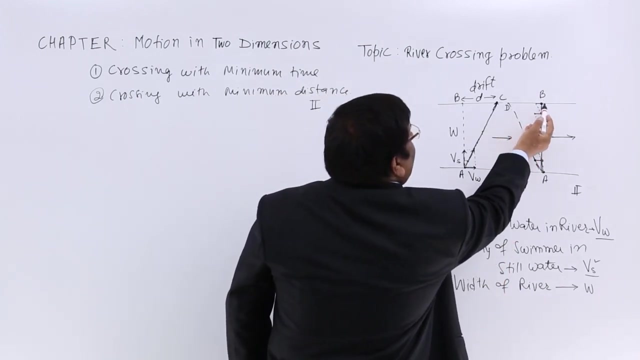 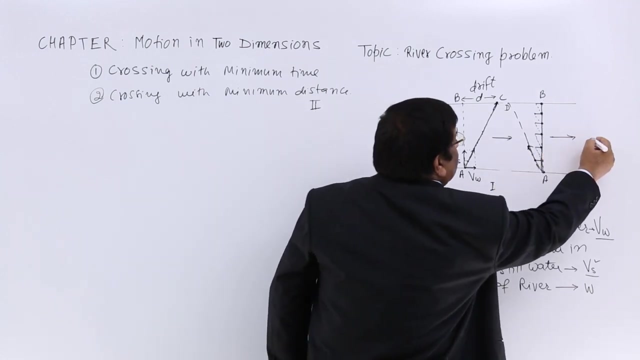 to cross the river and he wants to go just across his position, just across his position, with the minimum distance. how he should travel? answer: he must aim at a point on the upside. this is: water is flowing in this direction and water flows towards down. so here we will. 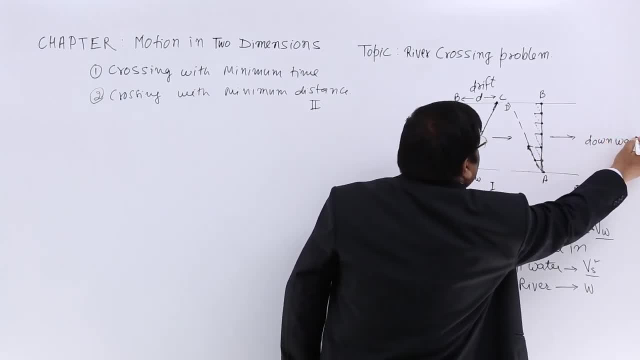 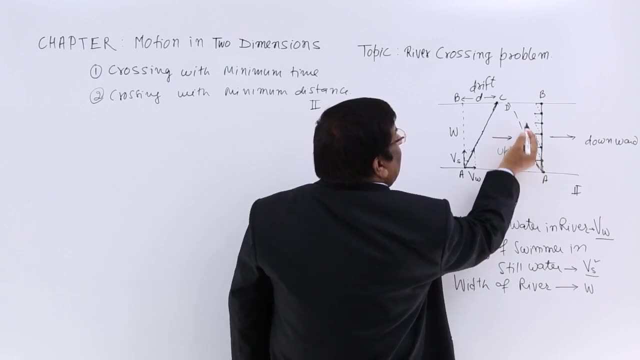 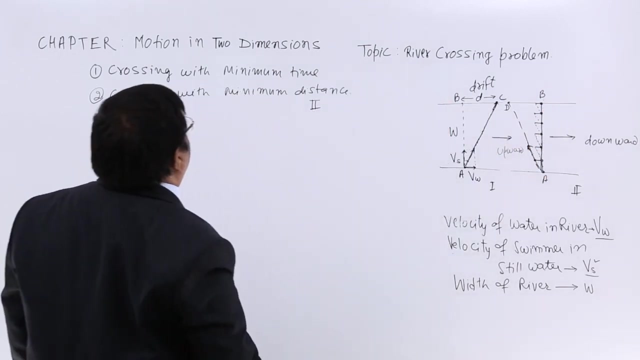 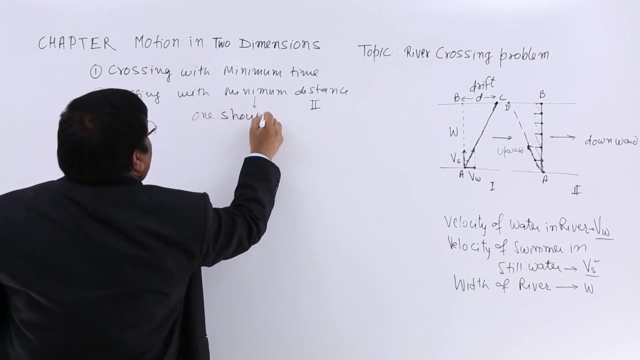 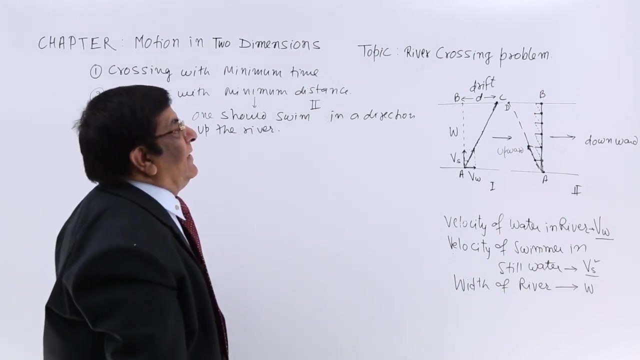 say downward, and this direction will be downward. So where he should target, he should target up the river. then he will be drifted to just point across it. so for minimum distance one should swim in a direction: up the river. ok, this is With the minimum distance now, in which case the timing is less and in which case the time 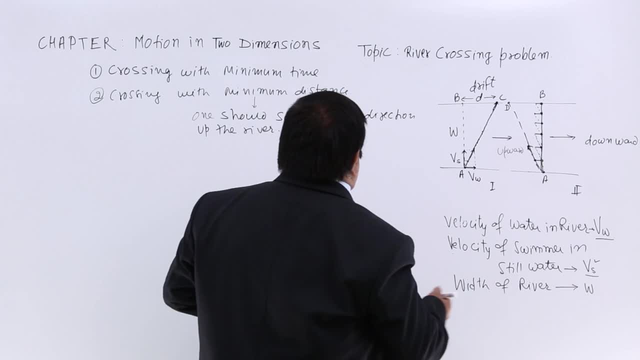 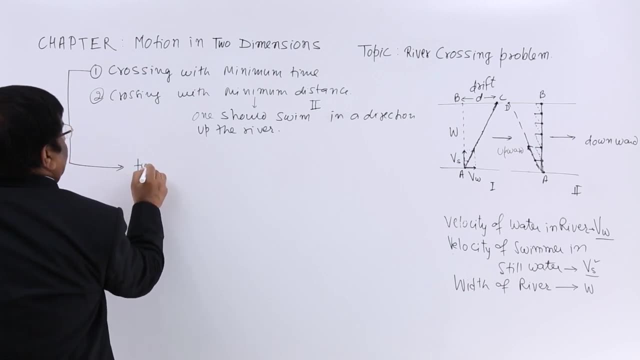 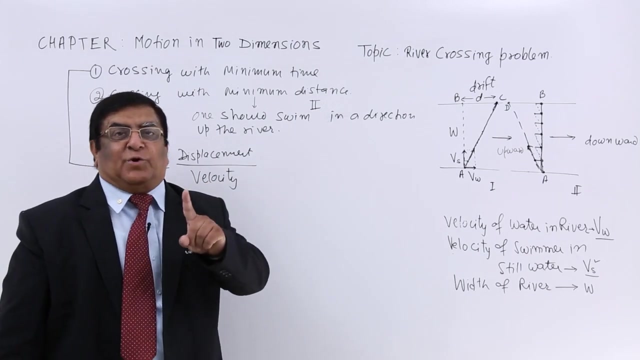 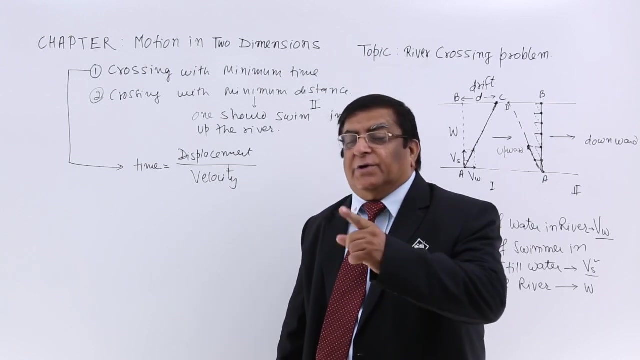 is more. see how to calculate the time. for the time, time is equal to displacement upon velocity. Ok, And one very important rule for the time is: when you are dividing displacement with velocity, make sure that both are in the same direction. this displacement cannot be divided with this. 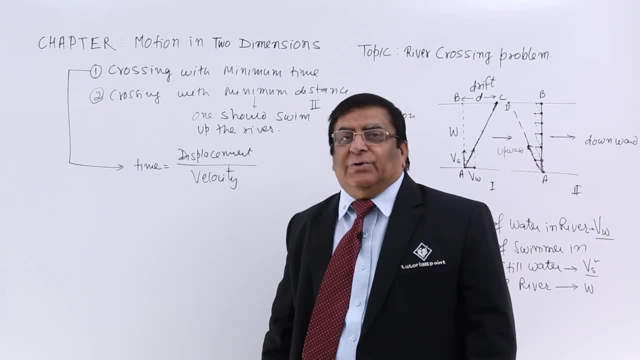 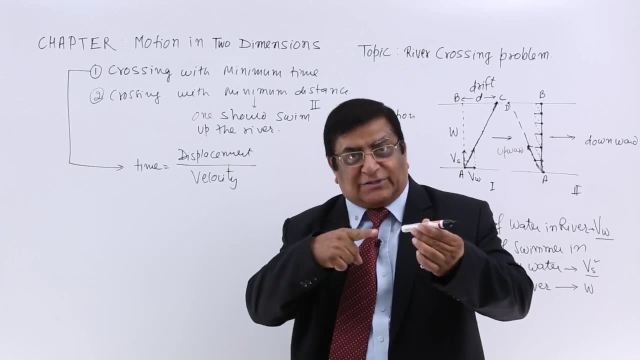 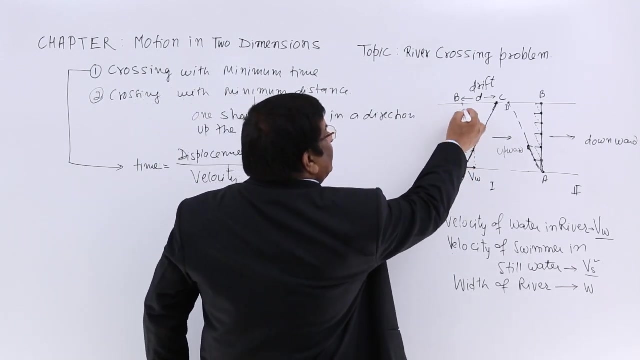 velocity. that will not give the time. So, in which ever path you want to go, if you want to go this path, then please calculate velocity in this direction. it is very logical. So here. Ok, If he has to cross the river, then let us take this path. how much is the length of? 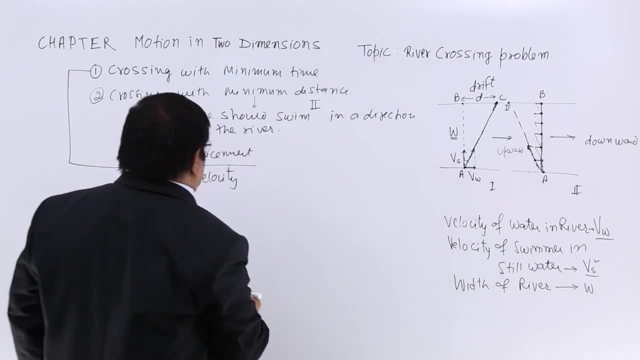 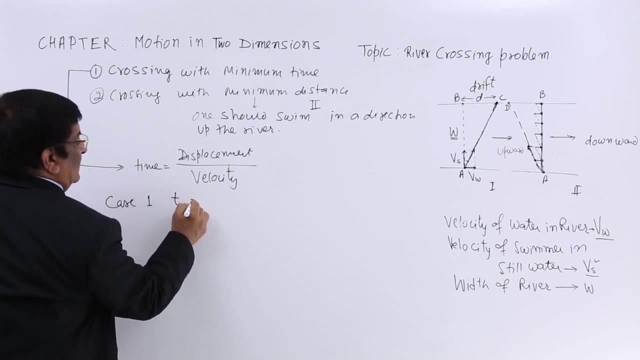 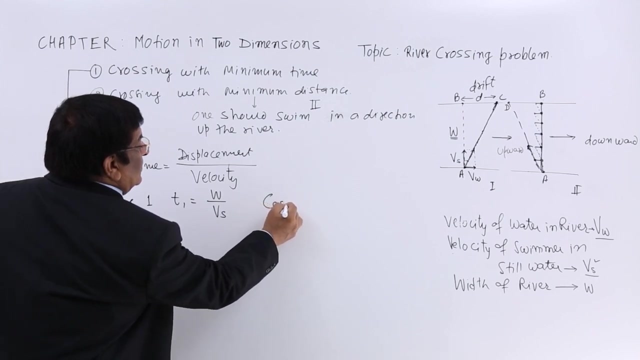 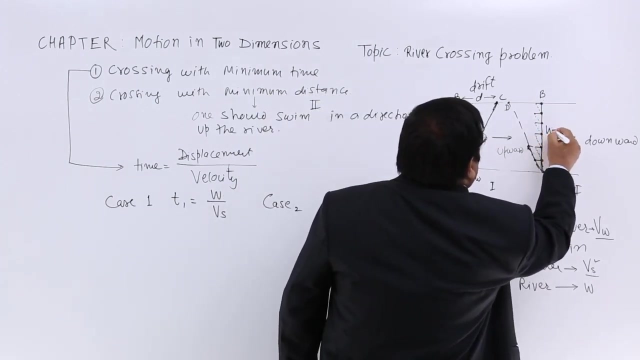 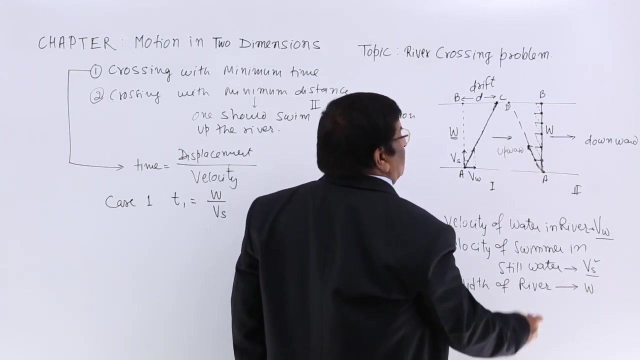 the path W. what is his velocity Vs? case 1, time is equal to displacement, W, and velocity is Vs. velocity of swimmer right. case 2, if this length is W, what is velocity in this direction? is it Vs? answer is no, this is Vs because he is swimming in this direction. 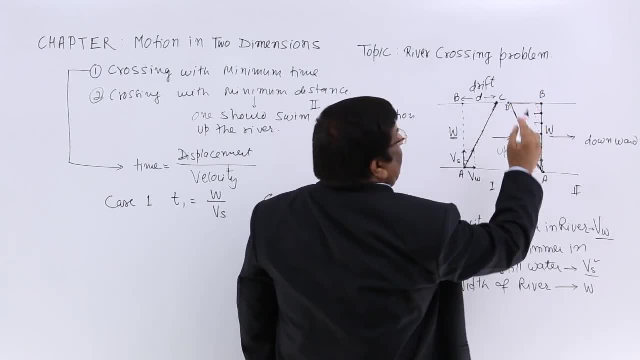 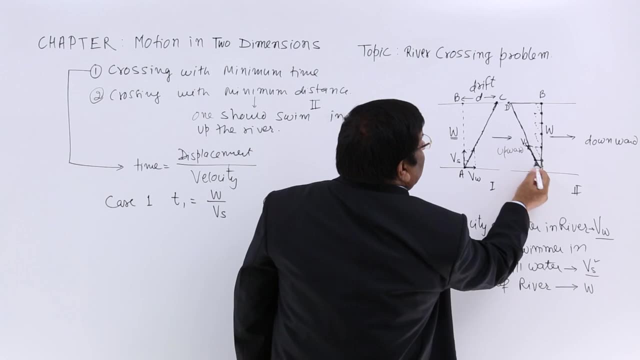 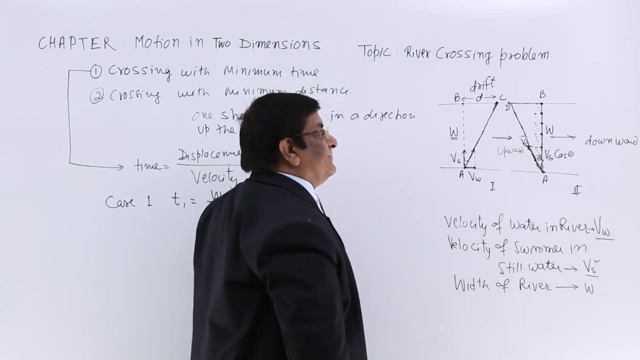 and this is W. This Vw will put it to this point. but the velocity in this direction is Vs. so what is the component of this velocity here? the answer is: component of this Vs. velocity in this direction is Vs cos theta. here is the angle: theta Vs cos theta in this direction. 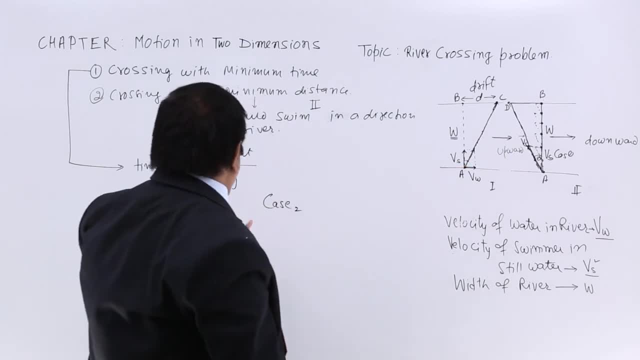 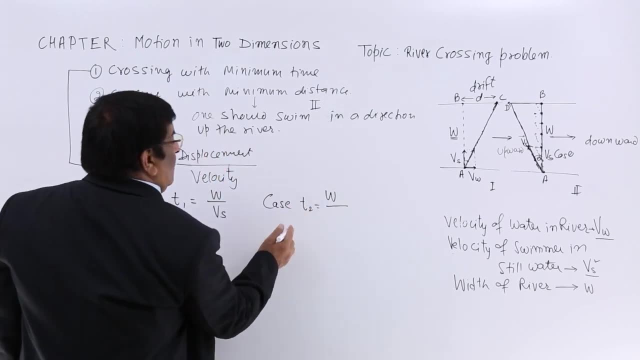 ok, So this is same W. ok, case 2, time 2 is equal to displacement W, but velocity is Vs cos, theta V2 is larger than T1, so in this case time taken is more than this case. but 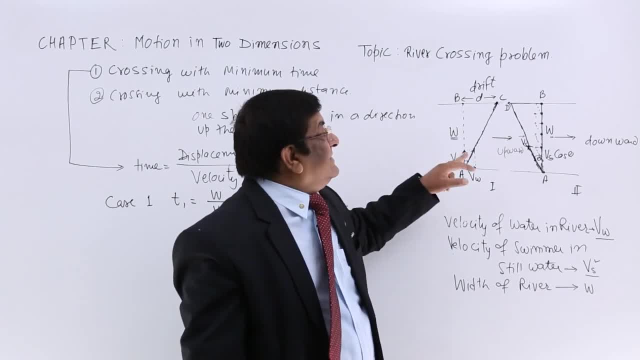 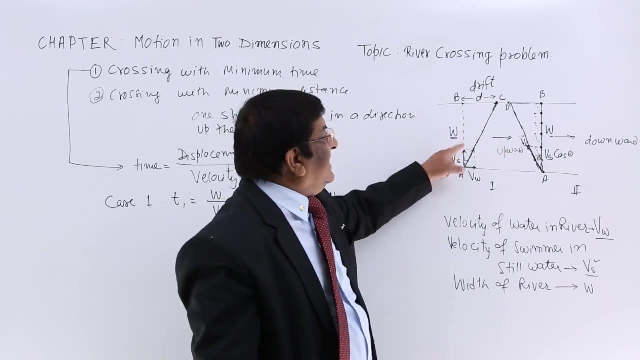 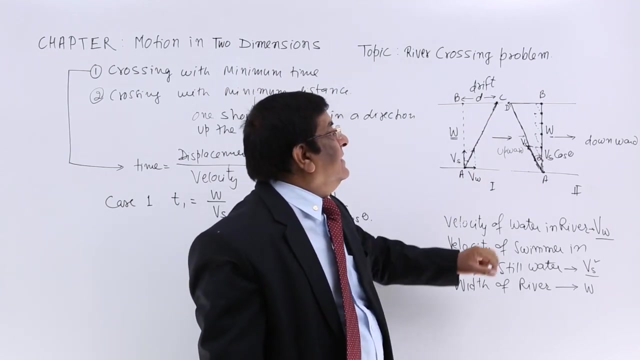 it appears that he is taking a longer time. no, he is taking a longer path, but he is going very fast. how do we know very fast? it is clear: it is Vs plus Vw. two velocities combine together. Vs plus Vw is this: 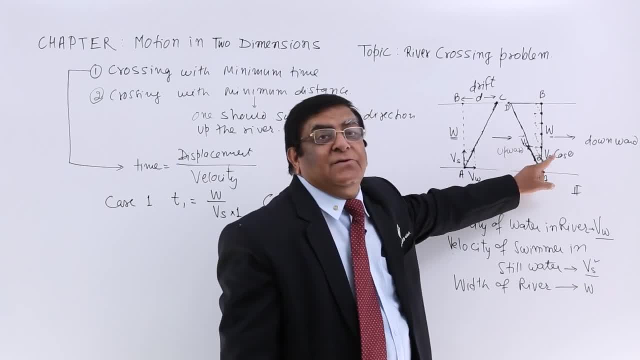 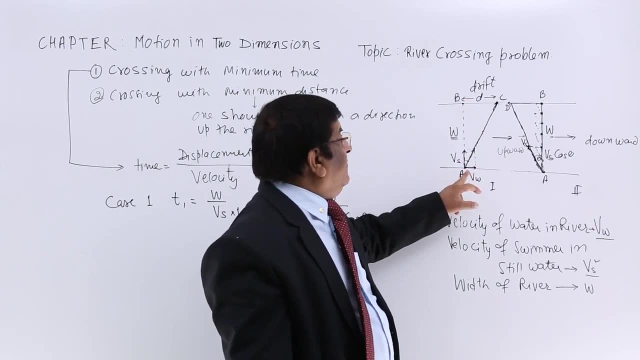 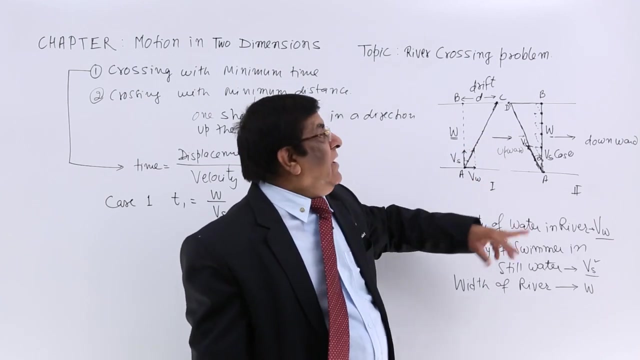 Now why. this is what a part of Vs Vs into a fraction, a smaller Vs like. if Vs is 4 kilometre, Vw is 1 kilometre, Ok, then this is root of 4 square plus 1 square more than 4, how much is this 4 into cos 30? 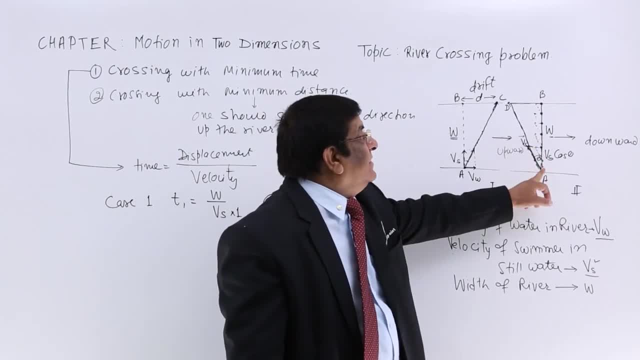 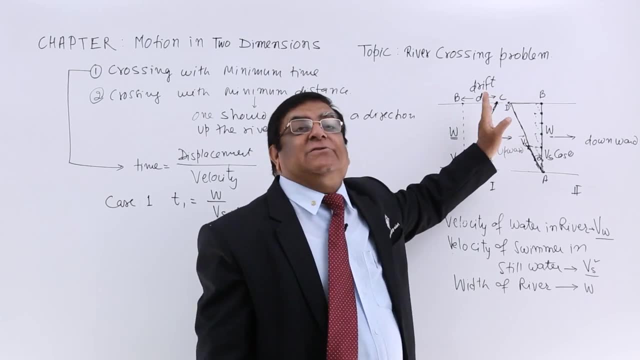 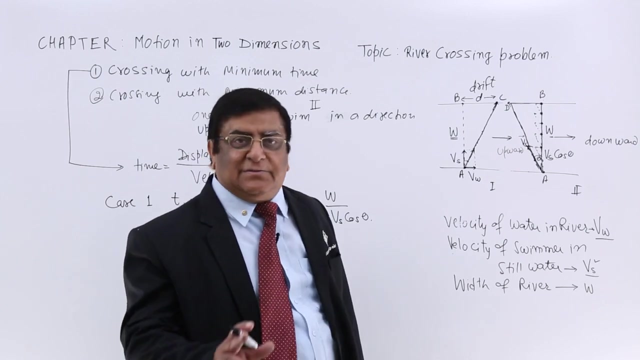 that will become 3.2.. So this is 3 velocity. here it is 5 velocity. So even if this longer, it will take a larger time. in this case it will take smaller time here because the speed is very fast. that is happened, So do not be misguided by the length. always remember: 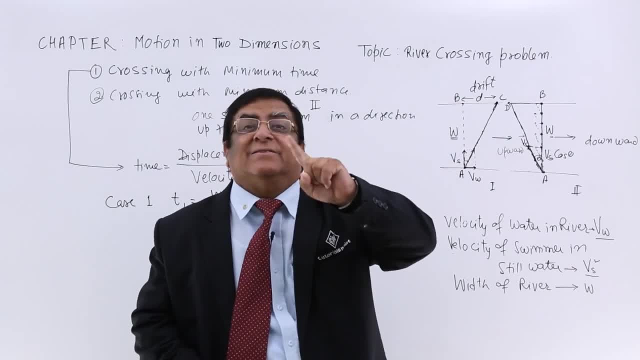 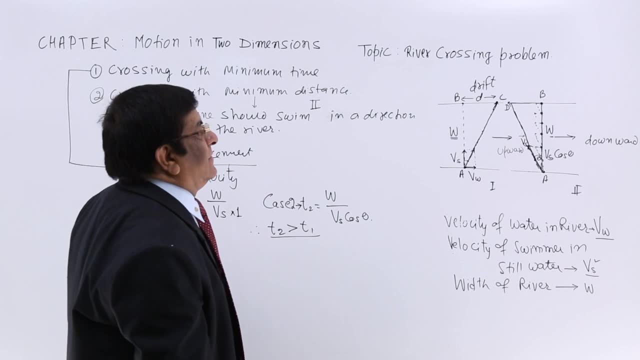 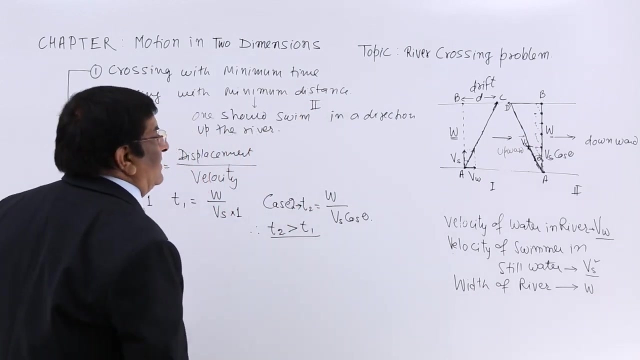 this is the way we can cross it in the shortest time, and this is in the shortest length. Then can we find out length here and can we find out time here? yes, both. the thing we study- case 1, case 1, T 1- is this: 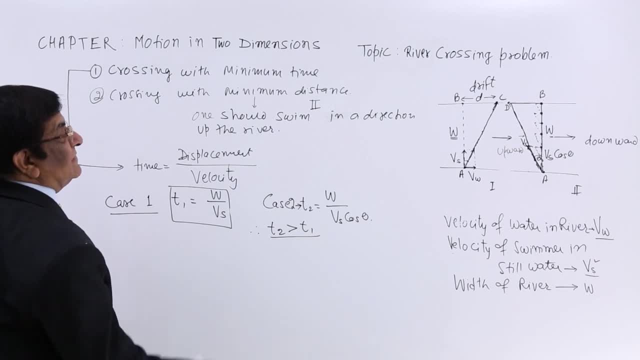 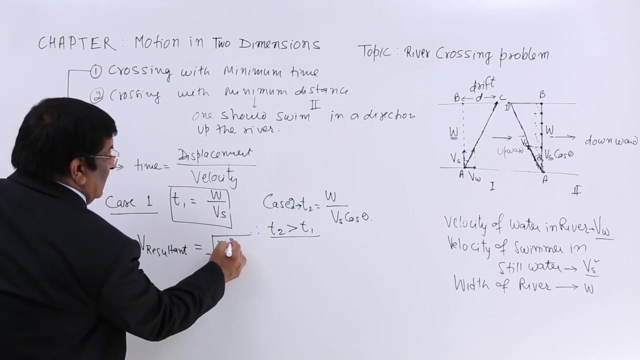 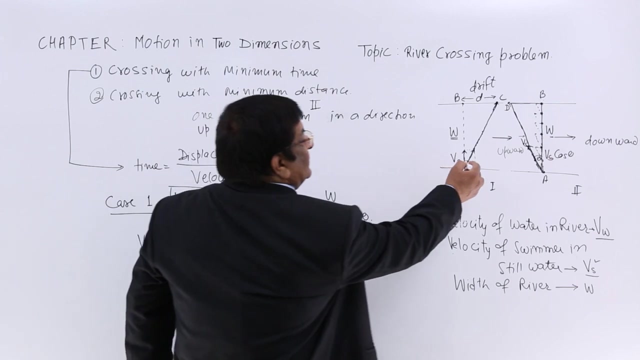 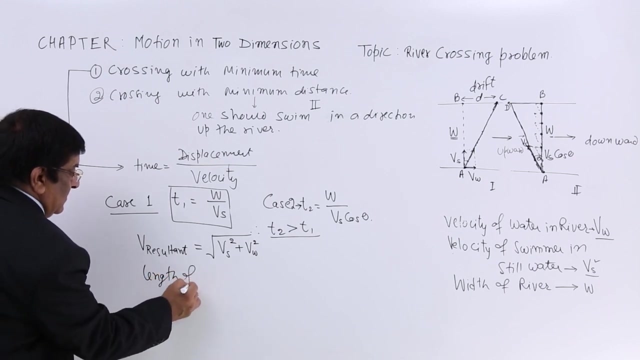 How much is the velocity, velocity resultant? Velocity resultant is equal to root of velocity swimmer plus velocity water. this is velocity resultant. this What is the length of the path? How can we find out? Answer is velocity multiplied by time. that will give us length of path There. 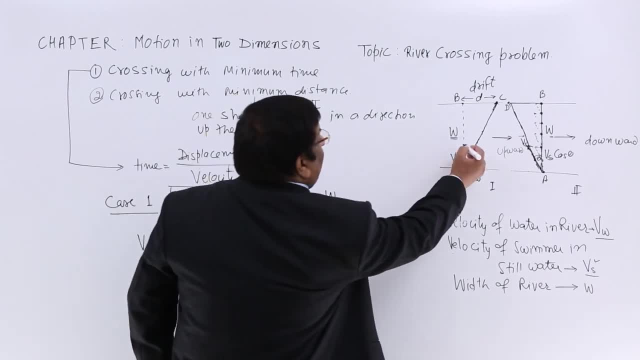 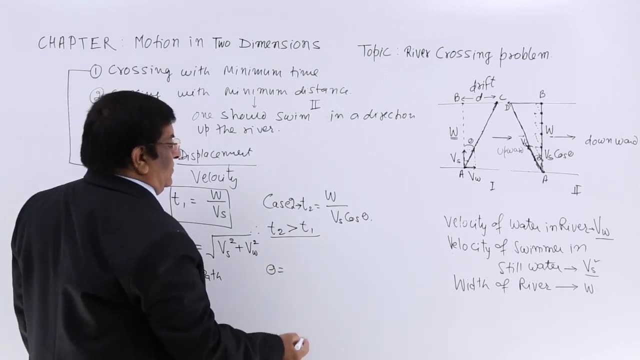 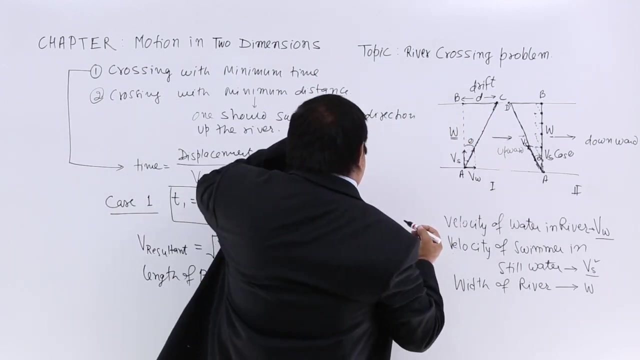 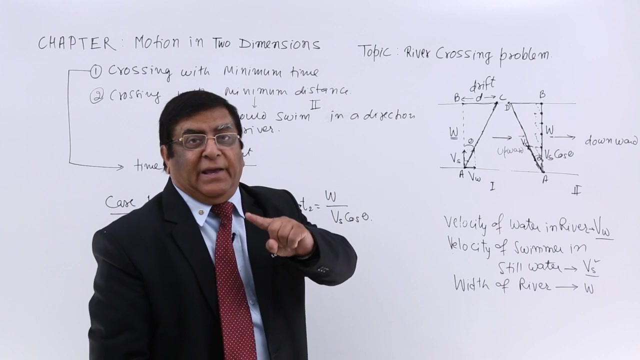 is another way to find length of path. what is this angle where he is drifting? Theta is equal to 10 inverse this. Ok, Let us make a triangle of velocities, triangle of velocity. we can make a triangle of velocities. 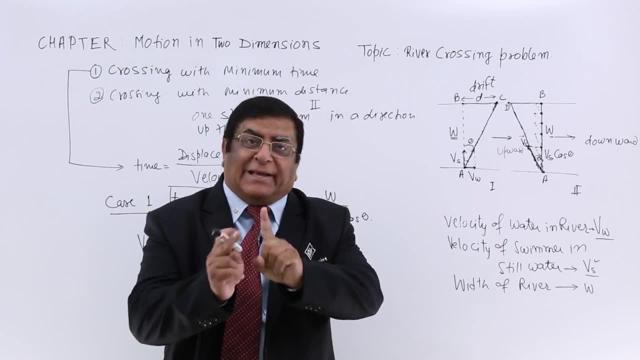 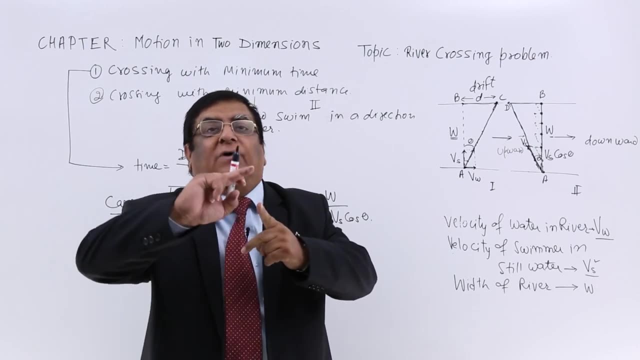 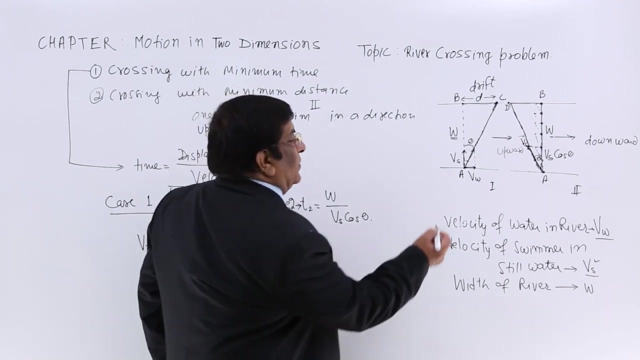 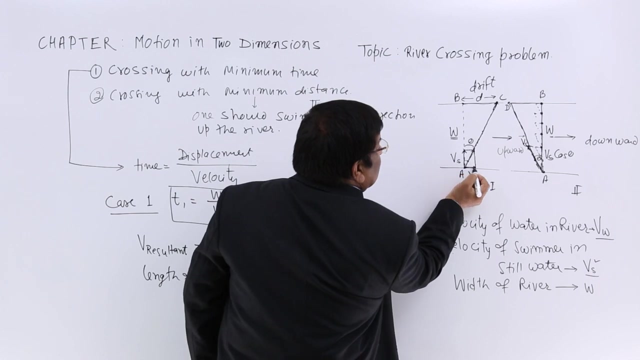 we can make a triangle of distances, but we cannot combine them right In one triangle. we cannot put one arm for velocity and one for distance. no, It has to be either all velocities or all displacement. So here, this is what this is what this is representing Vs. these are representing. 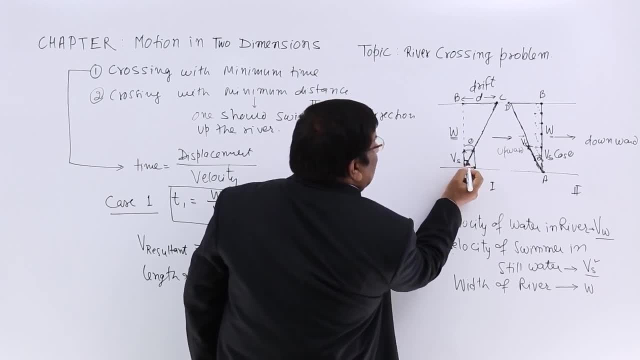 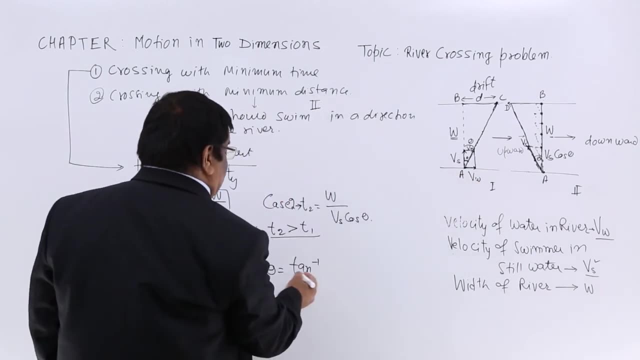 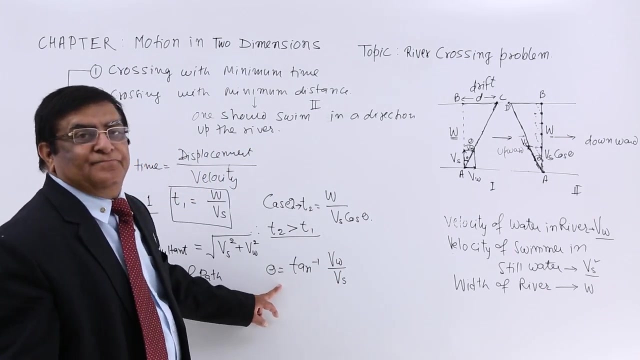 Vw, then how much is tangent of this angle? Tangent of this angle? theta is: here is Vw divided by Vs, Vw divided by Vs. this is theta. ok, That is this angle. Once again, you can g kerrière. 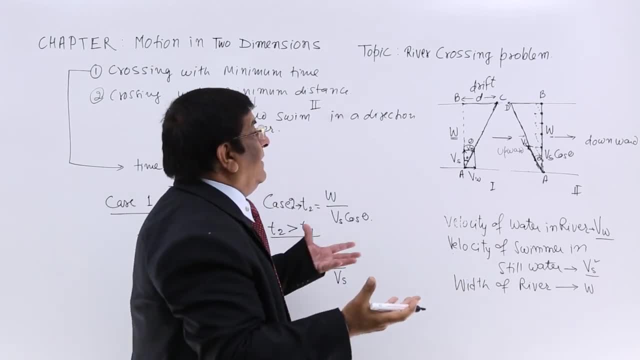 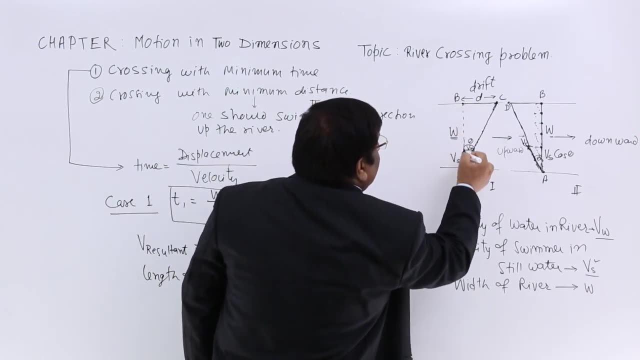 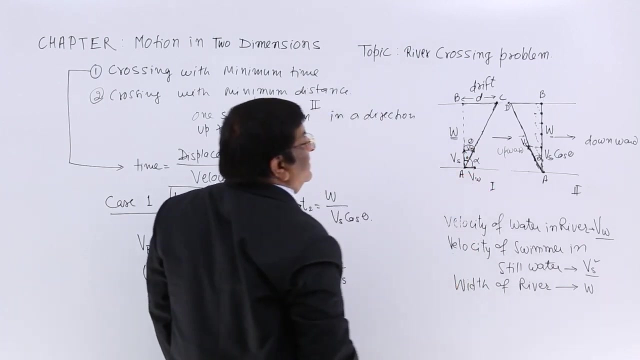 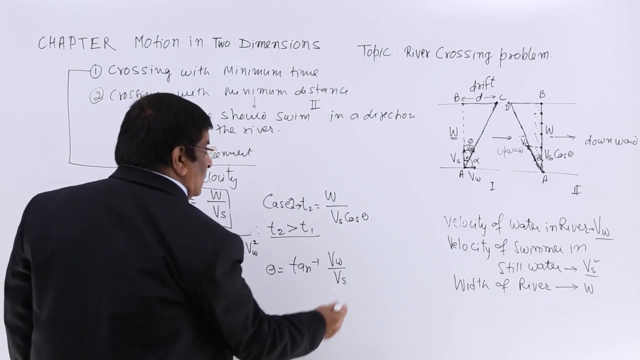 Now, how do you pronounce this angle? you will have to find out some way out. This angle is with reference to this line. if you want to show this angle alpha, then this is alpha, this is alpha. Tangent of alpha is equal to what? 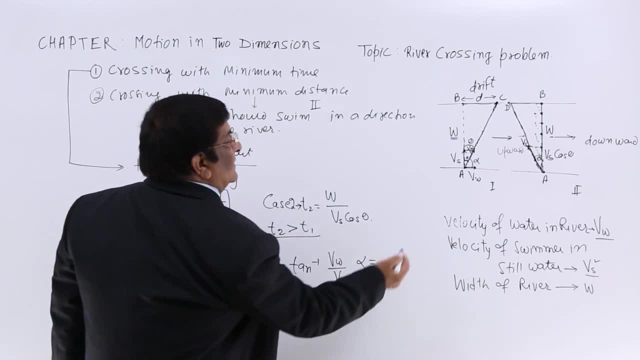 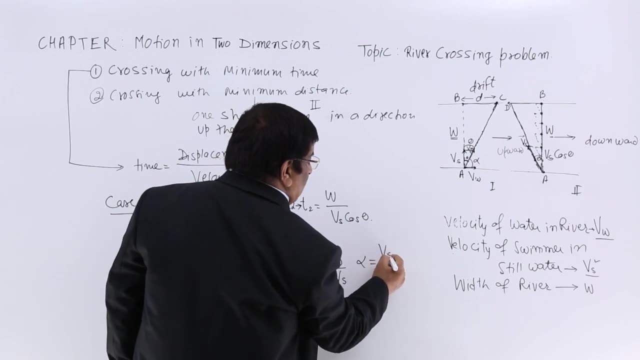 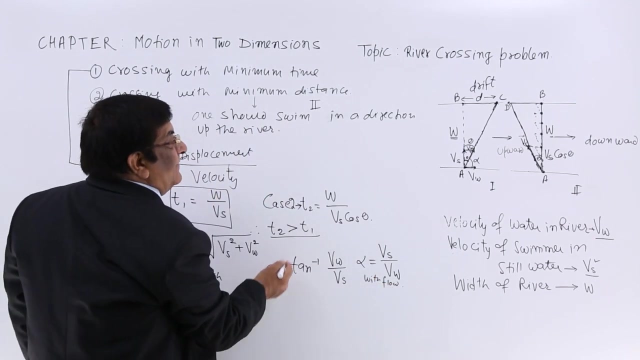 Tangent. tangent of alpha is equal to perpendicular upon base velocity of swim, divided velocity of water, And alpha is the angle with the water flow, alpha with flow. While it is very difficult to define theta, Theta is width, So it is difficult to measure it. So I think 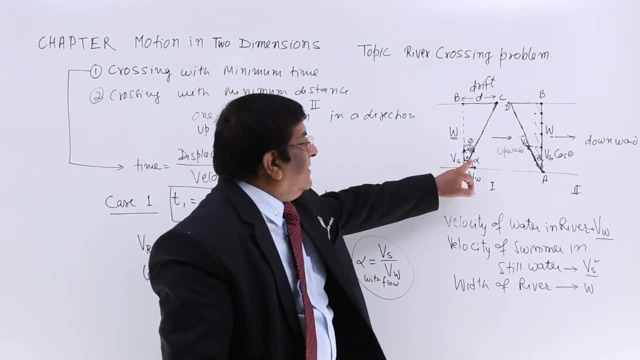 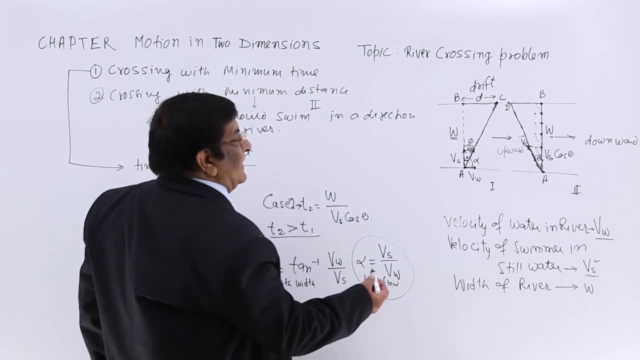 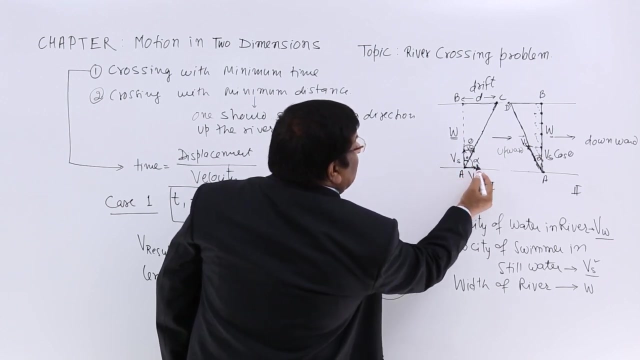 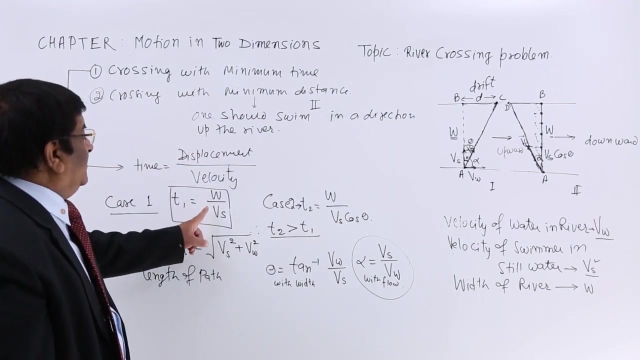 this is a better proposition: that alpha is tangent of alpha, is V s divided by V w, and that we can say: he should, he will go. he will go, making an angle so much with the flow. flow of water. other thing: how much time it has taken this much. that's right. another thing: 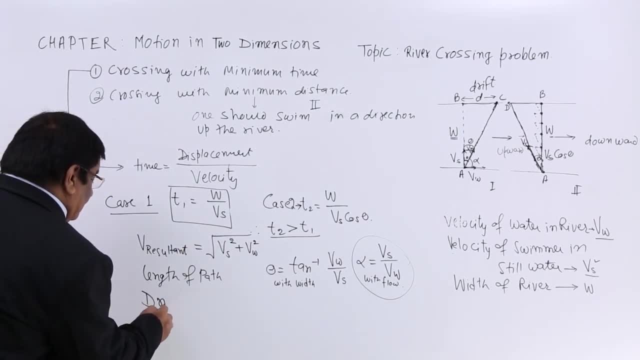 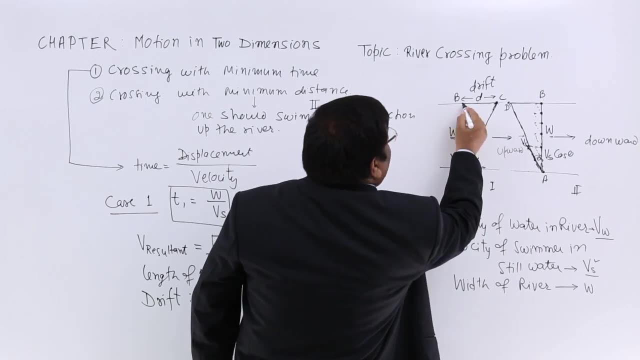 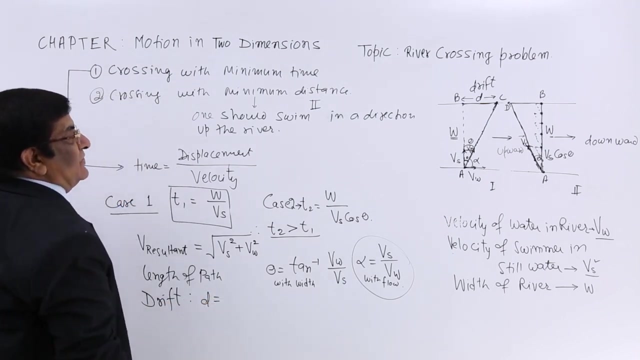 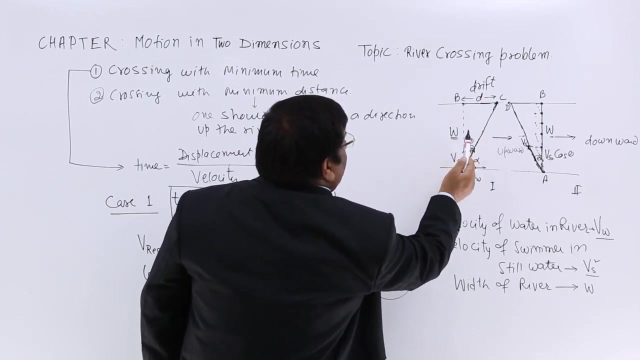 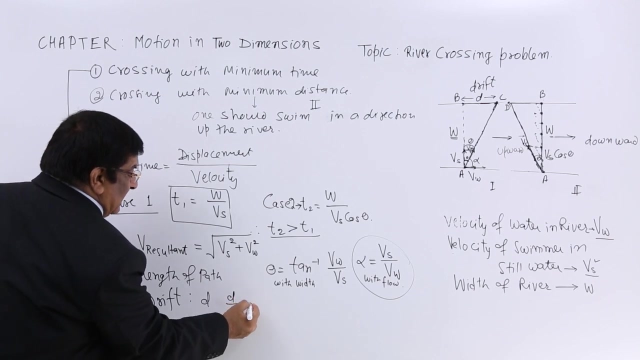 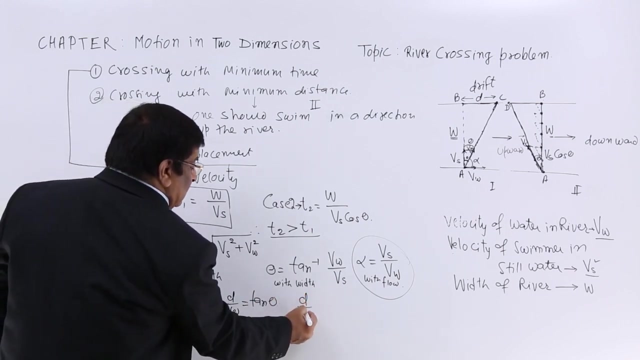 what is his drift in this case, this drift? he was supposed to go here but he landed here. so how much he has drifted. drift d is equal to this is w, this is d. so d upon w is tangent theta here, d upon w is tangent theta. that is d upon w is d upon w is equal to and tangent. 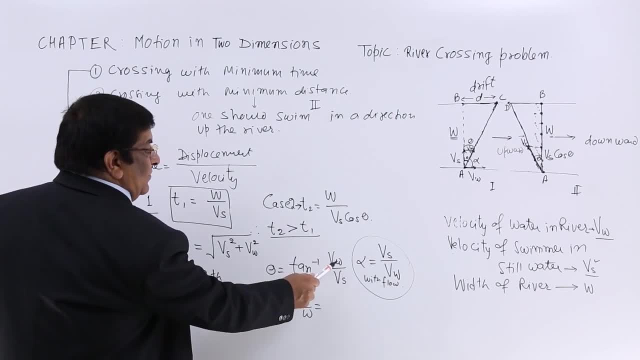 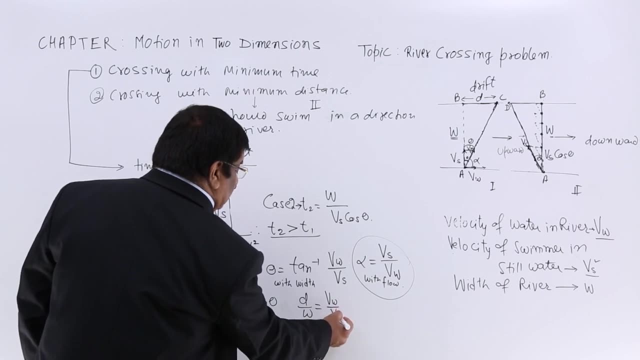 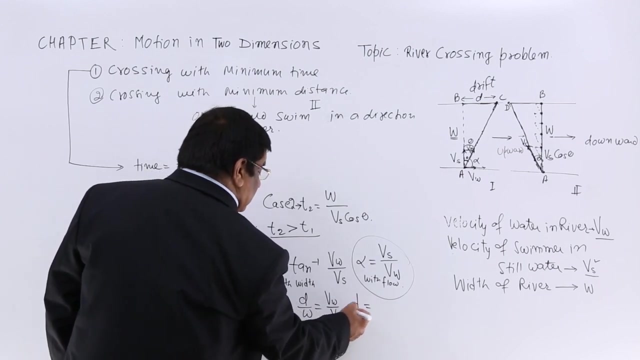 theta have seen theta tangent theta is equal to Vw upon Vs, So this we can write as Vw upon Vs. So how much is d equal? to Answer drift: d is equal to width of the river multiplied by width of the river, multiplied by velocity of water divided by velocity of swimmer. This 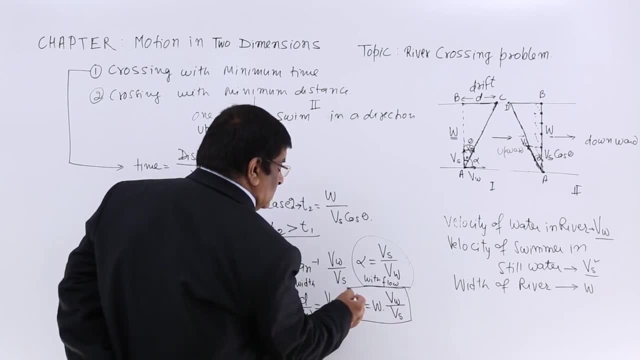 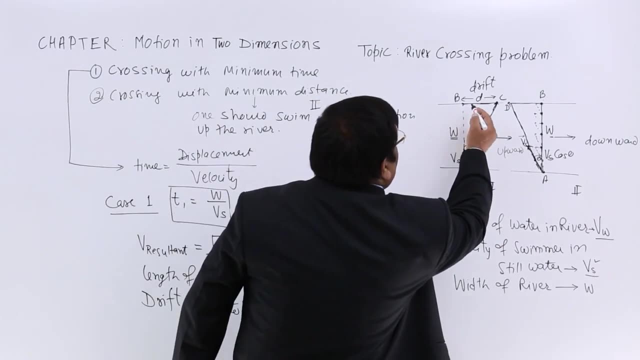 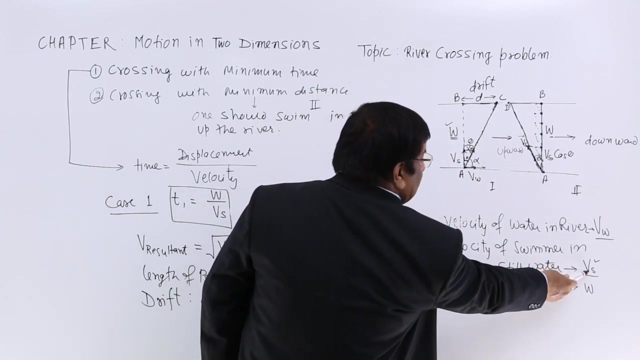 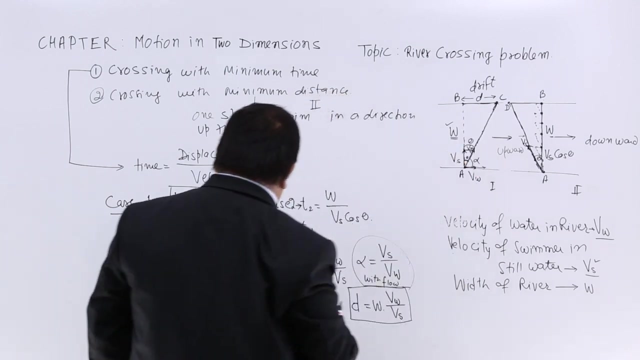 is drift. This is how we calculate the drift. So now we have calculate, we have what was the given quantity. The river has a width w. the swimmer can swim with Vs. What is the drift? This is the drift. What is the time to cross? Time to cross w. 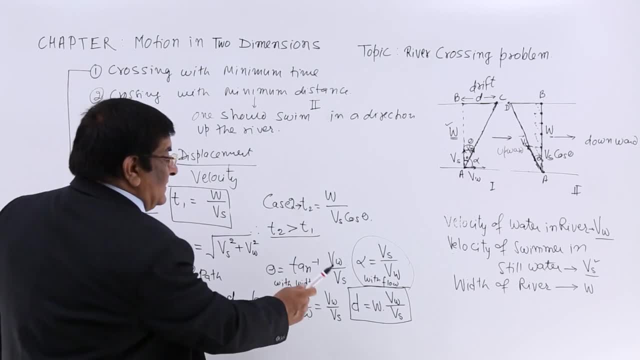 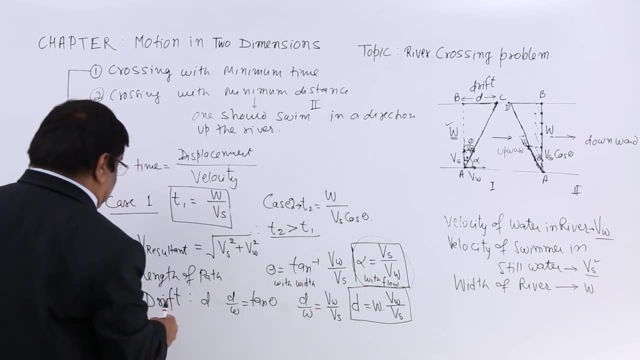 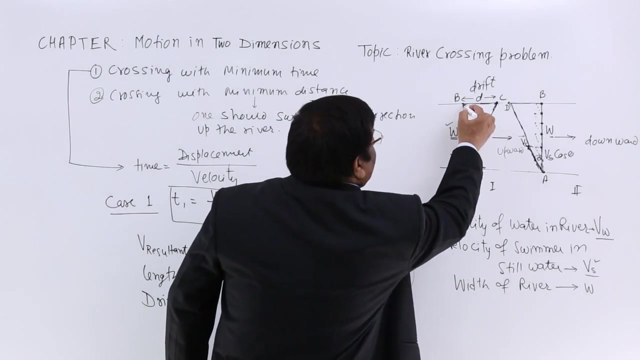 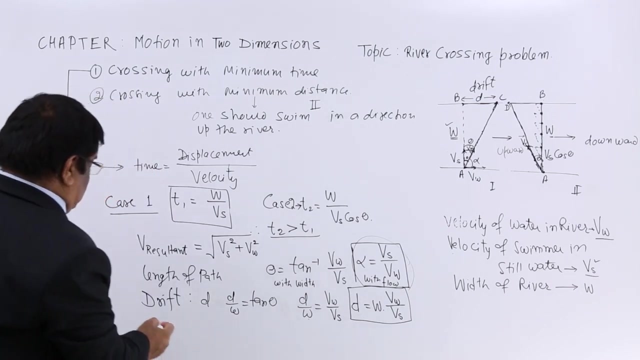 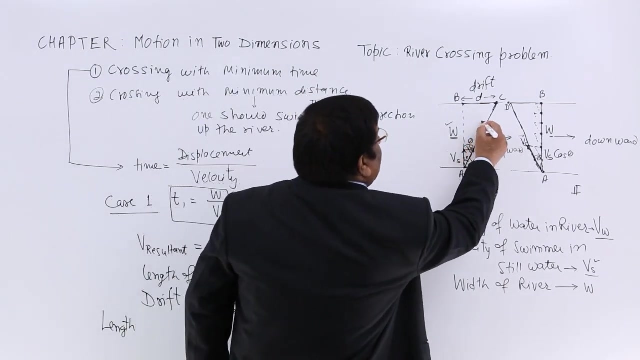 upon Vs. This is one answer. this is drift answer and this is at what angle he has gone. and this is: where is the length of the path somewhere. Length of the path is this: If this is w, Then length of the path length. Let us write this: length of the path: L. Now you can make. 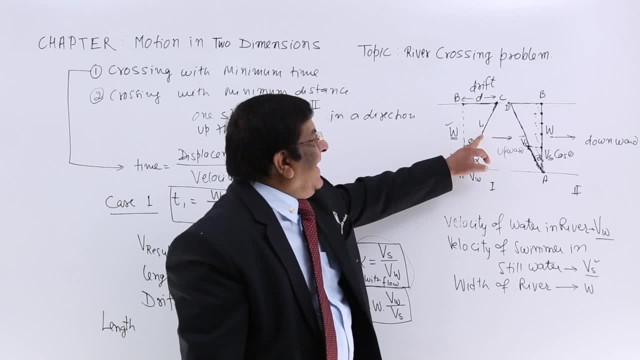 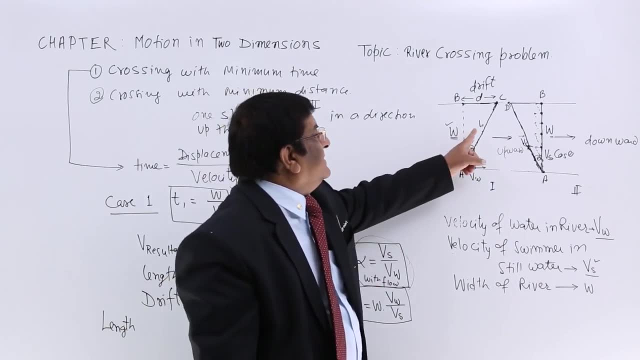 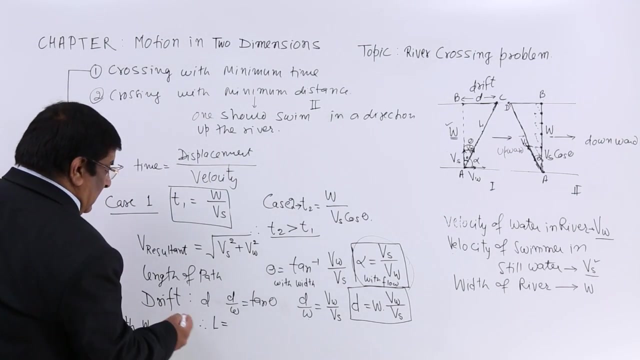 an equation that w upon L is cos theta, w upon l is cos theta. or you can say: this length is equal to square of this. this hat e square of this. You can say W upon L. that is right. L is equal to L. goes here here. 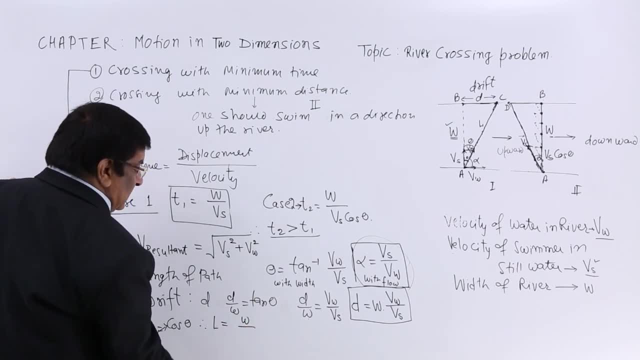 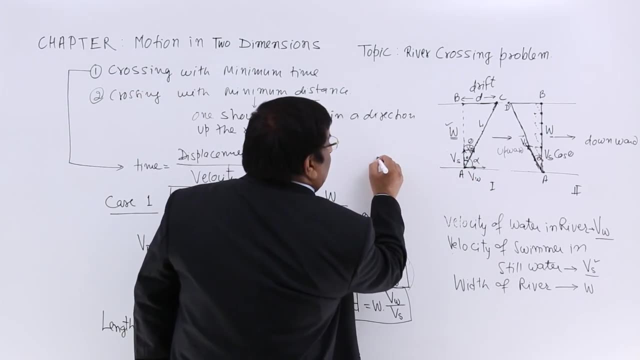 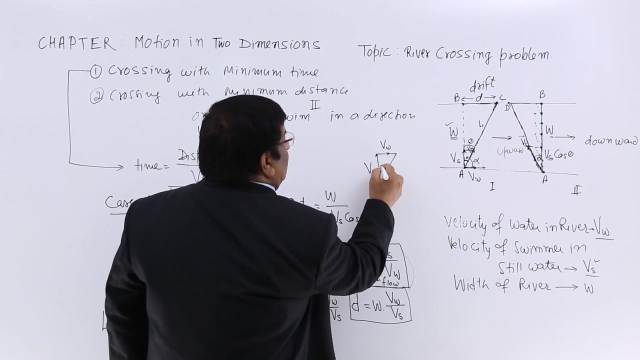 it is W upon cos theta, and you can always find value of cos theta from this smaller angle. what is the smaller angle? It is this, this is Vw, this is Vs and this is the direction. and for theta Now, what is cos theta here? Cos theta here is: yes, this is cos theta, this. 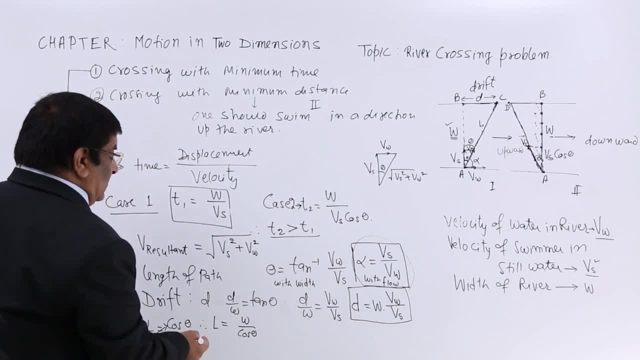 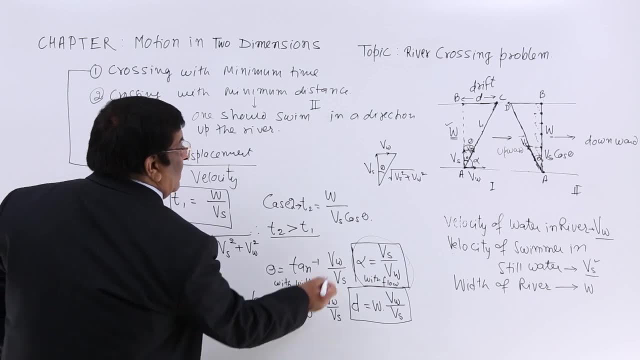 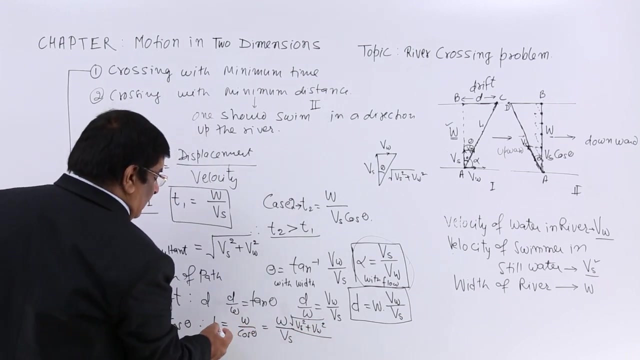 upon this. So L is equal to W upon cos theta, and this we can write as W upon for cos theta: Vs. Vs divided by root of root of Vs square plus Vw square. This is, we have found the length which so W is given to us. 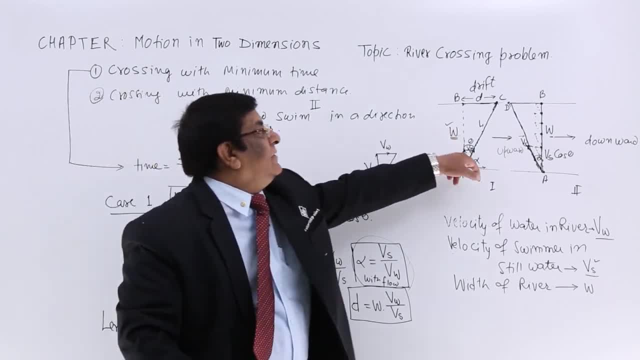 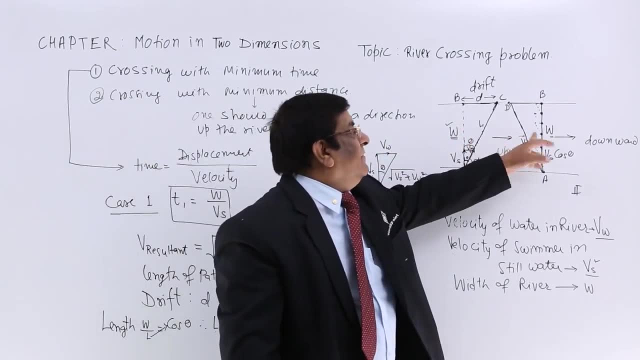 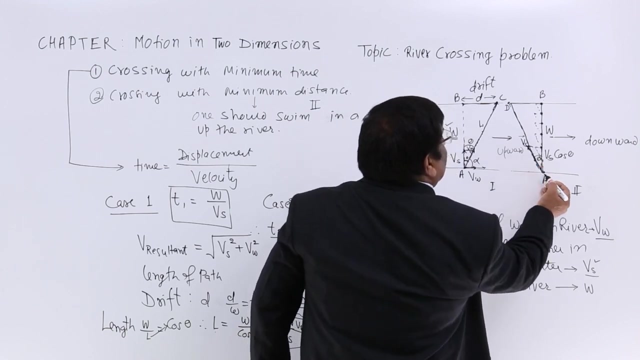 Vs and Vw is given to us. this is the length of this path. So everything you have calculated here, similarly you can calculate everything here. so that was the case I now in case II: what should be this theta where he should angle it? 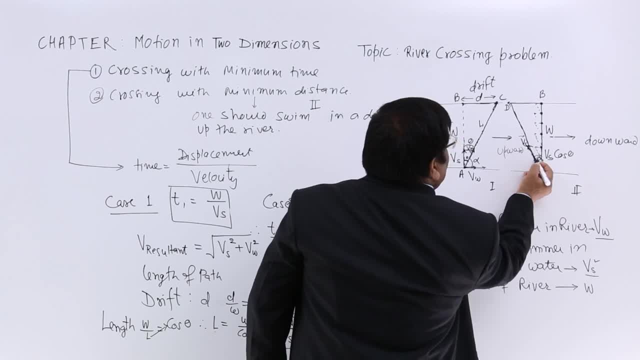 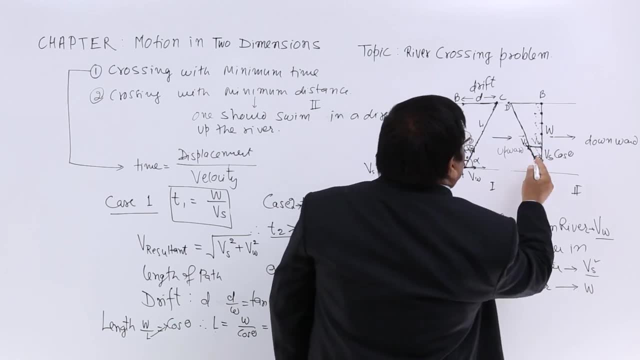 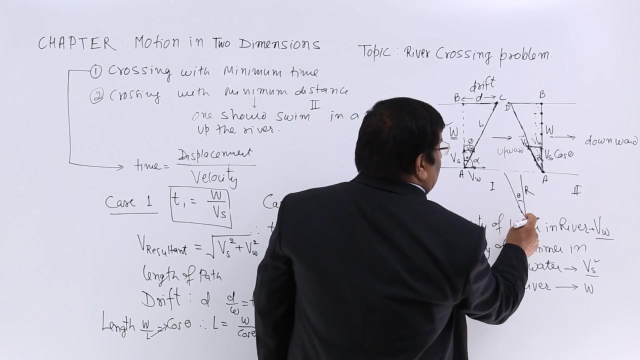 The answer is: this is his velocity Vs, this is velocity of water, Vw. where is this triangle? This triangle- I make it like this- Here is theta. He has to go this direction. That means this is resultant. If this is resultant, this is one component, Vs and this is other component. And what is this component? This is V of water. 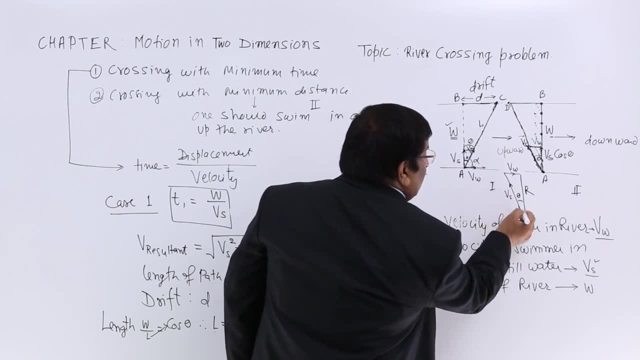 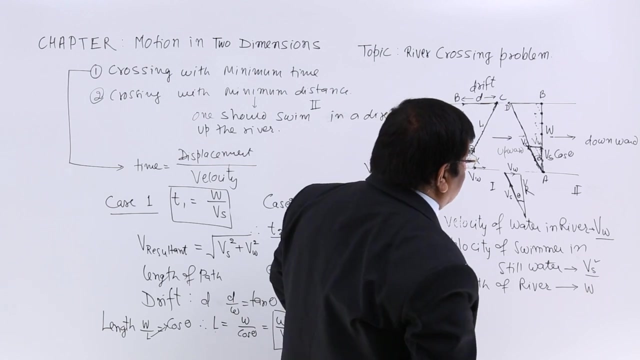 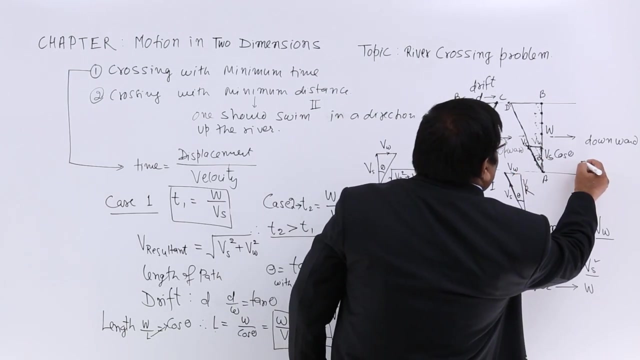 Why Velocity of swimmer, velocity of water, is velocity resultant. This is theta. So now can you tell me a relation for theta. What is Vw upon Vs? Very clear, it is sine theta. So what should be the angle theta? here, Theta is equal to sine inverse Vw. 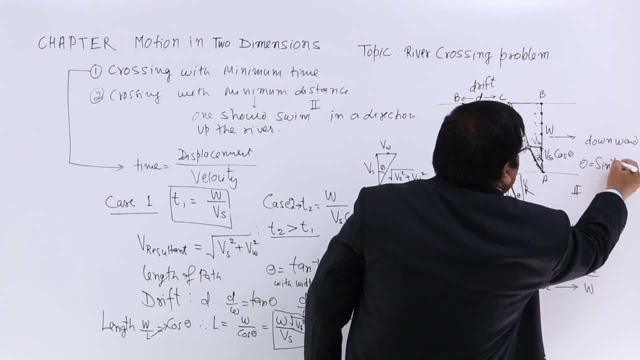 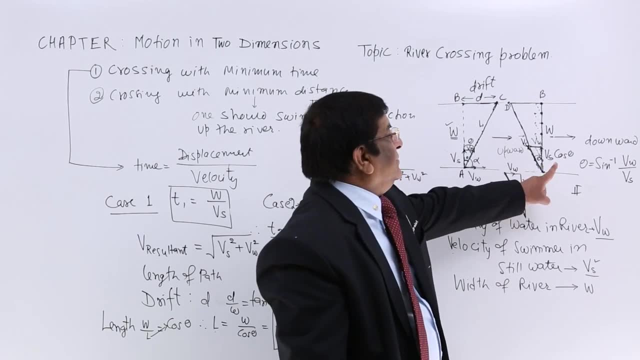 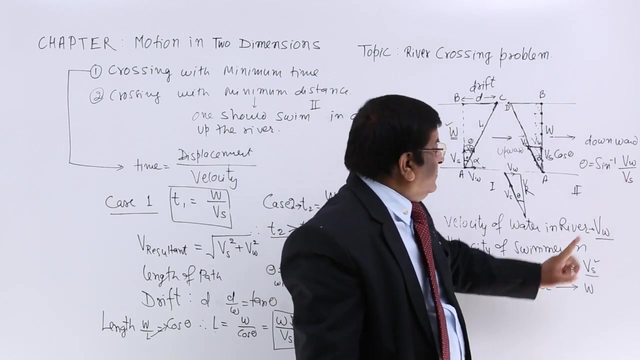 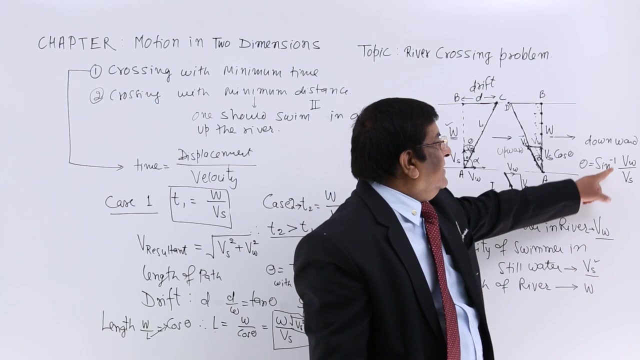 Vw upon Vs. Sine inverse Vw upon Vs. This is this theta He should maintain. If he is maintaining this theta, then he is going to reach just across it And it is very easy to maintain. We know the velocity of water and we know our capacity to swim. Just divide the two. That will give the sine theta. 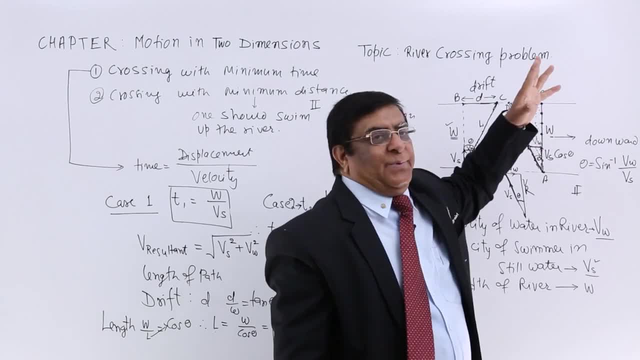 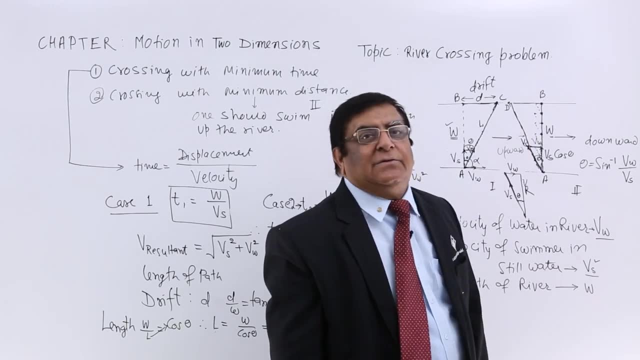 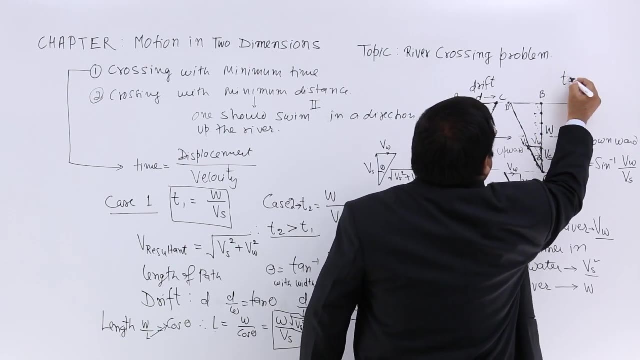 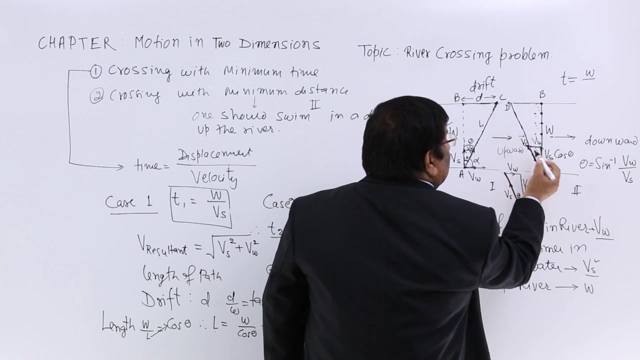 And with that angle he should go, Then he will reach. So you got to know this theta calculated How much time it is going to take. That is very easy Time. What is this displacement? W, W? What is this velocity? We do not know, Because this is Vs in this direction, Vw is in this direction. We do not know it, But we can calculate it. 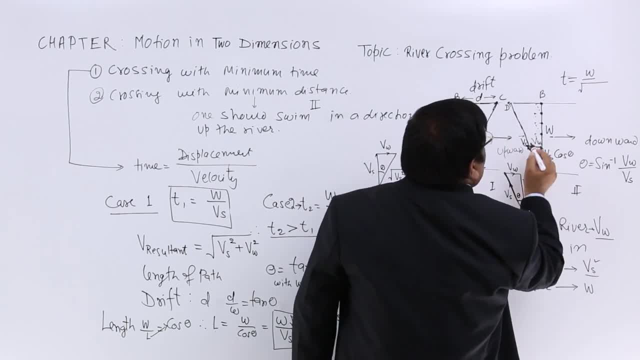 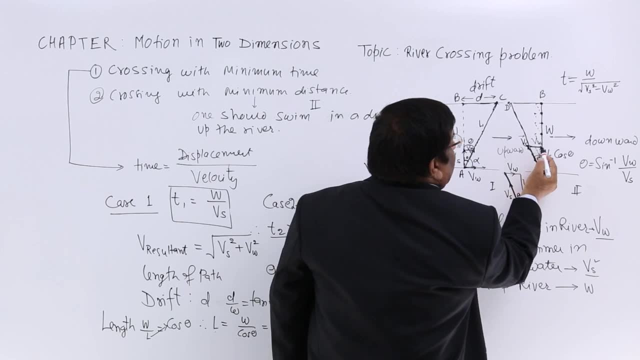 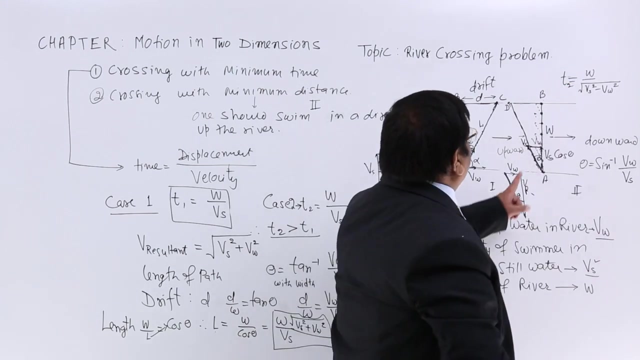 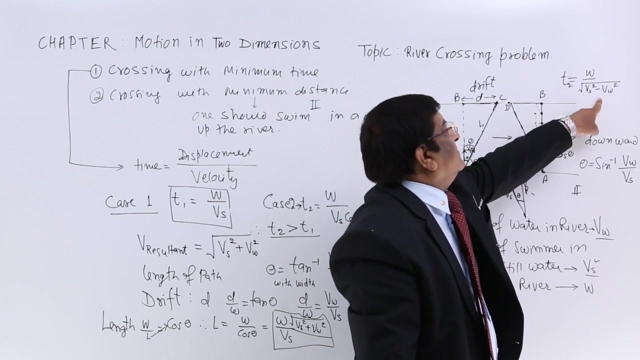 This will be root of Vs square minus Vw square. Vs square minus Vw square Is this: This gives us time. Now you understand what is the theta. Now you understand how much time it is going to take. It is going to take this much of time. 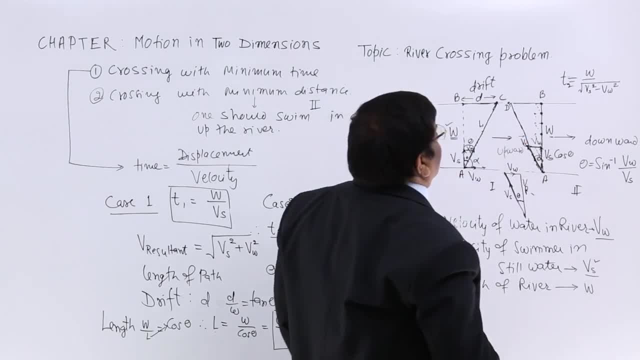 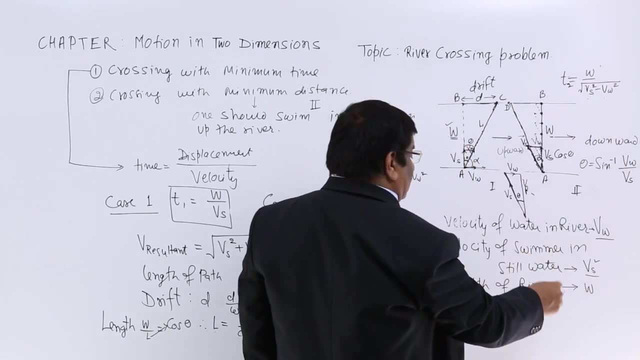 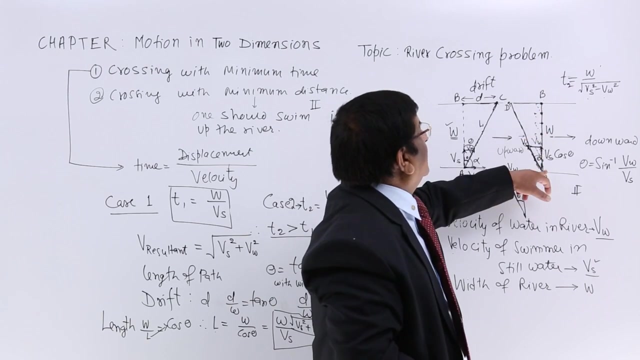 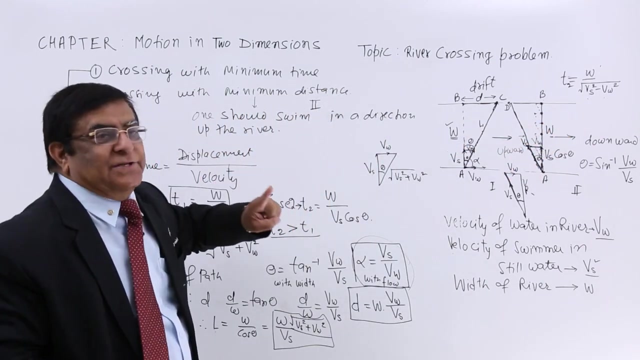 And this time is definitely larger. Okay, So this, this, this, These three are the given quantity to us. So this is theta, This is this Time, so much, And these are the things which we needed here. So this is analyzing both the cases, Please remember. 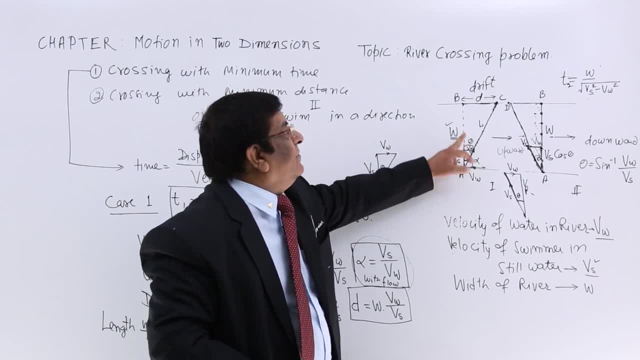 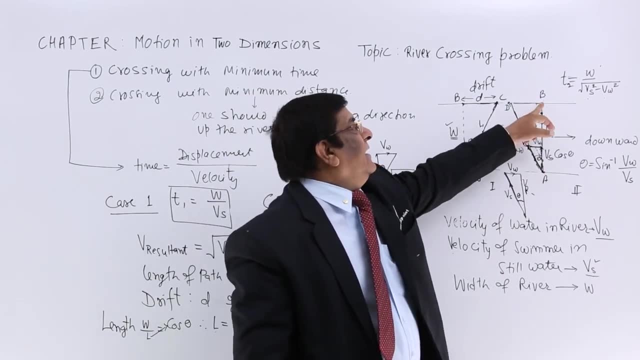 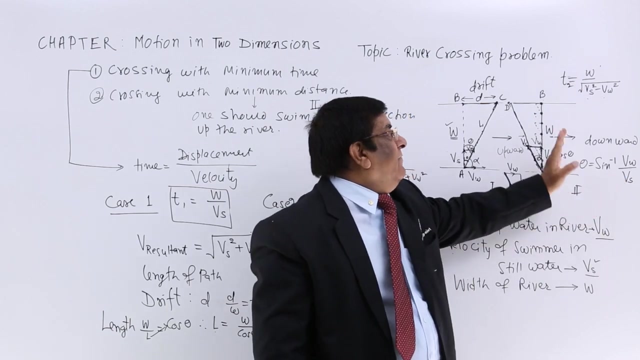 For shortest time he will try to swim straight and he will land up after a drift. Shortest time, Shortest length he must reach here. For that he will make an effort in reverse direction by an angle sin inverse Vw by Vs. 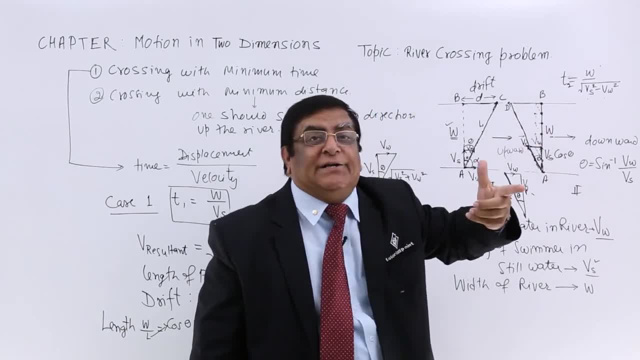 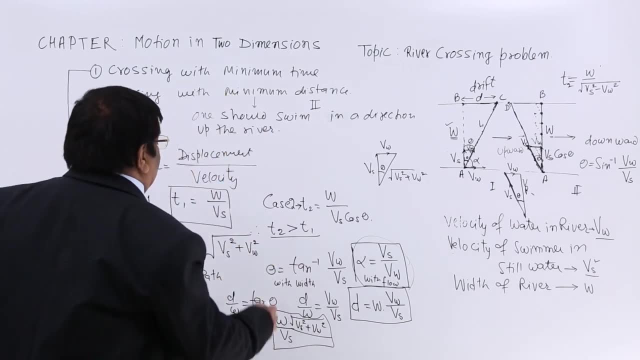 Then only he will land up here, But he will take a longer time. How much is that longer time? W upon Vs square minus Vw square, While in this case it was a smaller time. W upon only Vs Here Vs minus Vw.